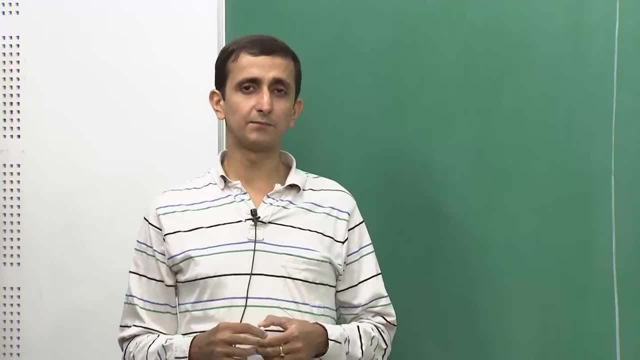 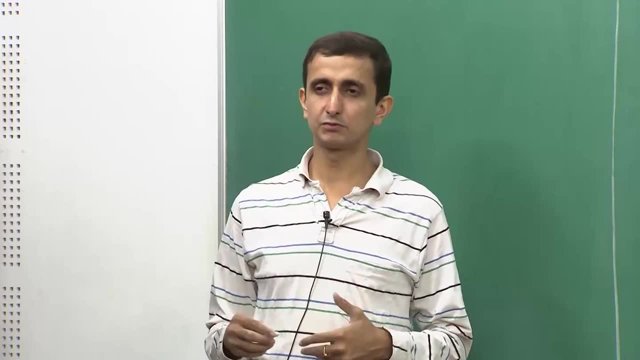 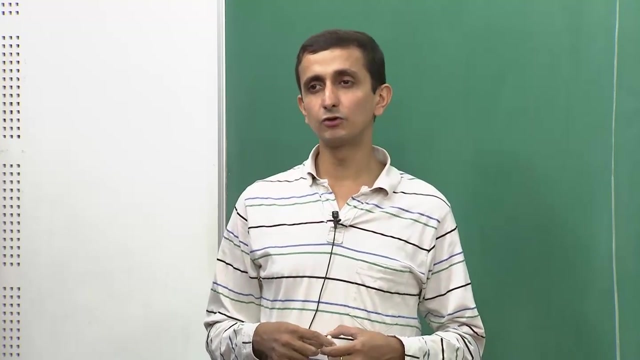 So far we have seen several class of languages and for the past few lectures we have been, our focus was mostly on the set of undecidable languages. We saw various undecidable problems and last lecture we saw a mechanism which we can use to show that languages are undecidable. 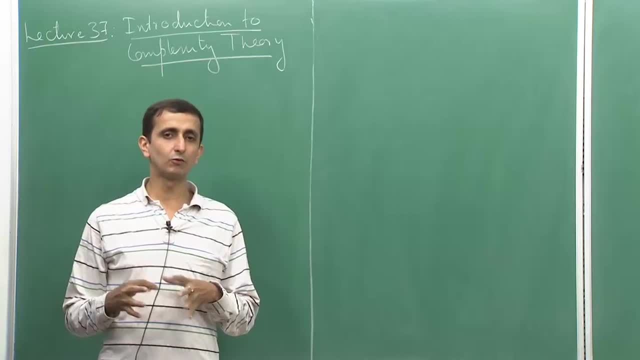 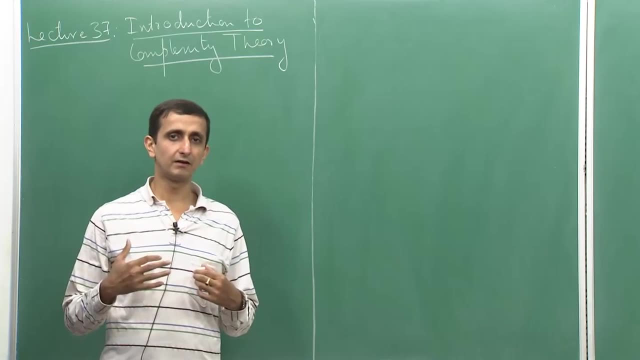 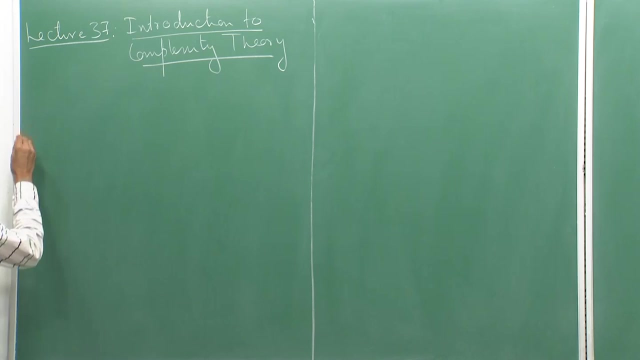 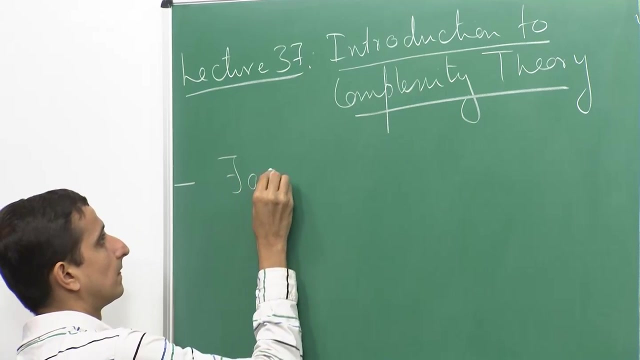 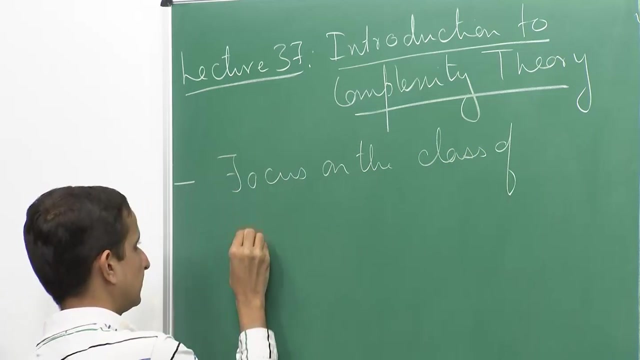 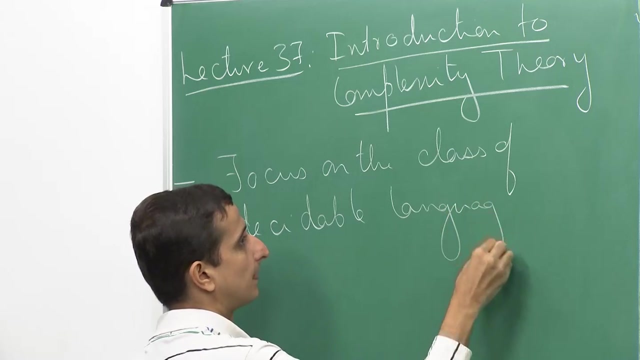 But from now on, we will only focus on the set of decidable problems and we will give a finer gradation, we will give a finer classification of this set of decidable languages. So, as I said, that we will focus on the class of decidable languages. 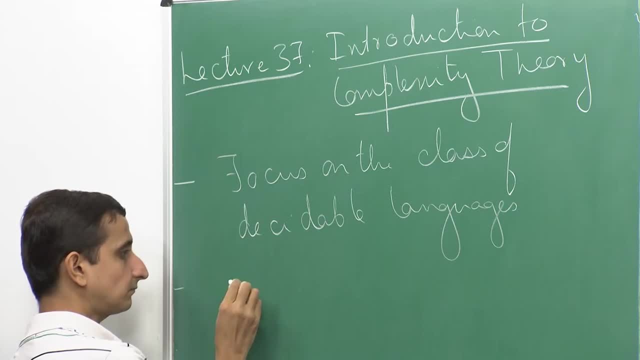 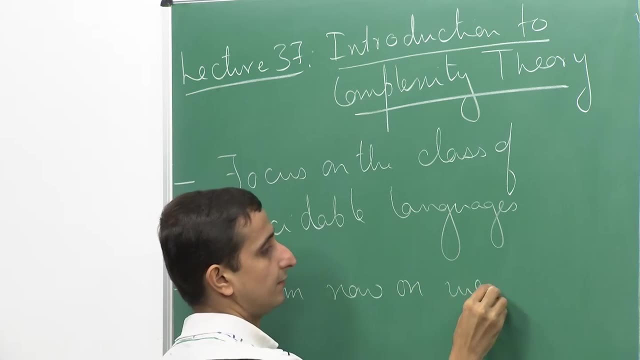 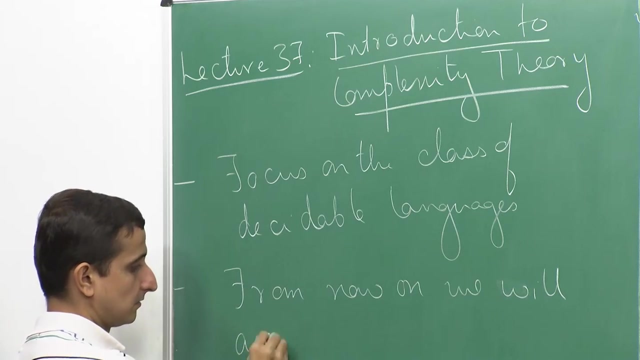 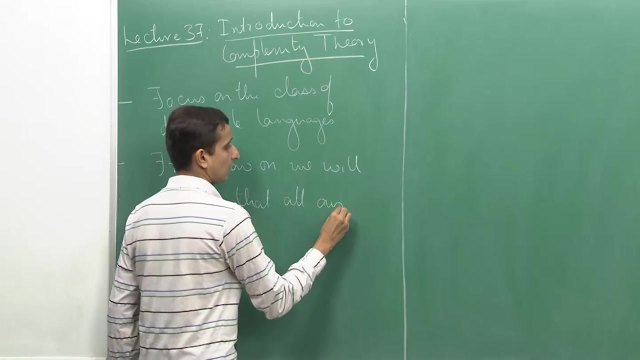 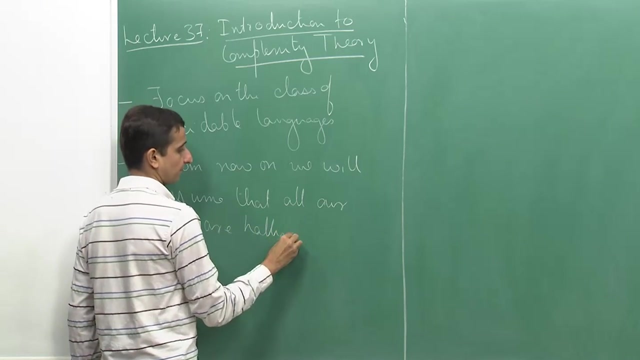 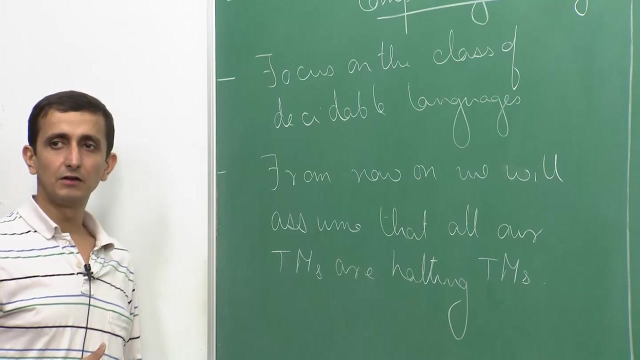 So therefore, from now on, we will assume that all our turing machines are halting turing machines, Of course, unless otherwise specified. if I specify something else, then of course we will assume otherwise. But we will assume that the setup of each set of decidable languages 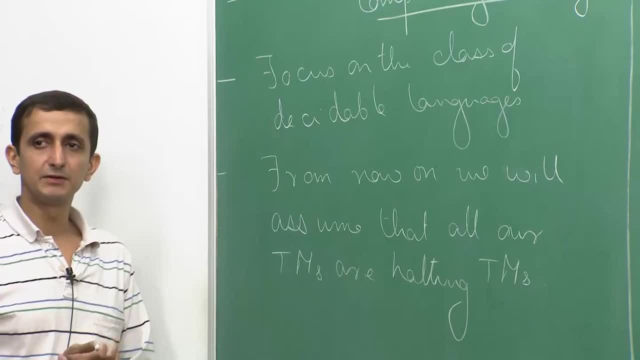 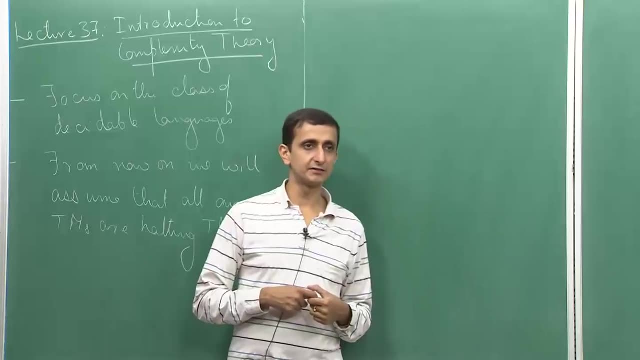 is in the conjecture that the set of decidable languages are undecidable. So this is what? otherwise, but by default, we will assume all the Turing machines are halting Turing machines. So what do we study in complexity theory? What are the kind of questions that we want to address? 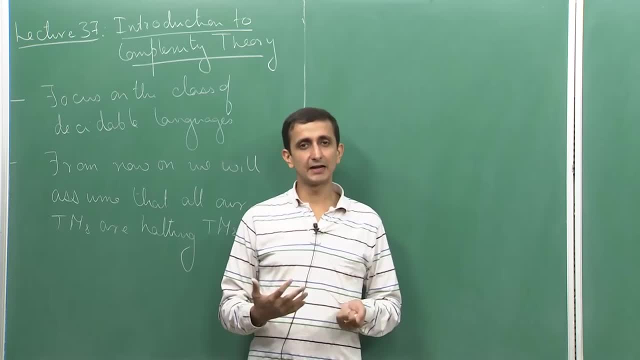 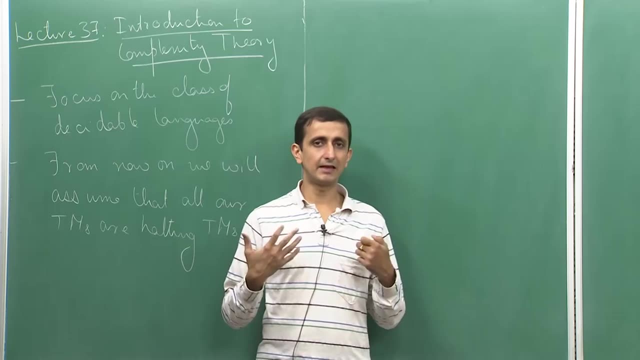 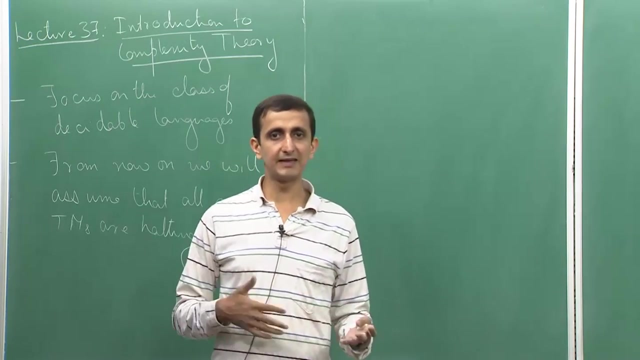 So first, what we will do is that, within the class of decidable problems, we will classify them based on the amount of resources that a particular language uses, or a particular Turing machine of a language uses, to reach its answer. So resources can be many things. resources can be time, they can be space. 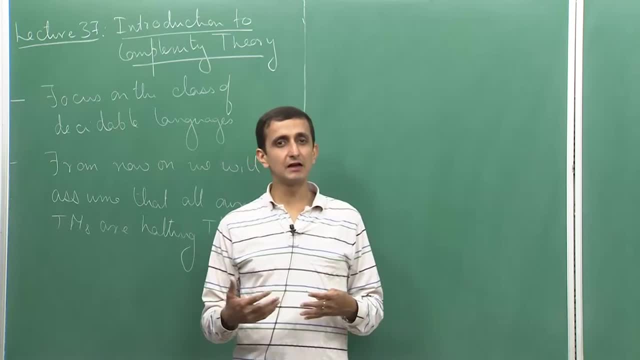 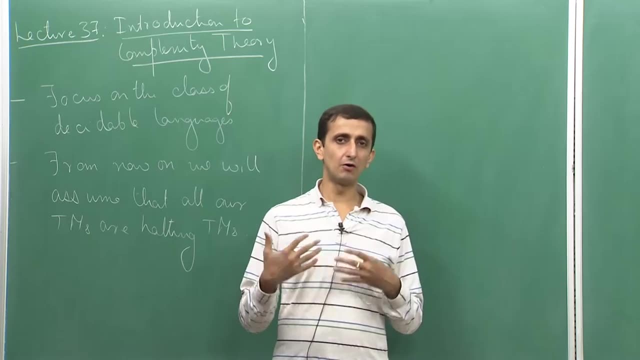 So if you are looking at, let us say, time as a resource, then we will try to see how much time does it take for a Turing machine to come up with its answer and, depending on the amount of time, we will classify language into different classes. 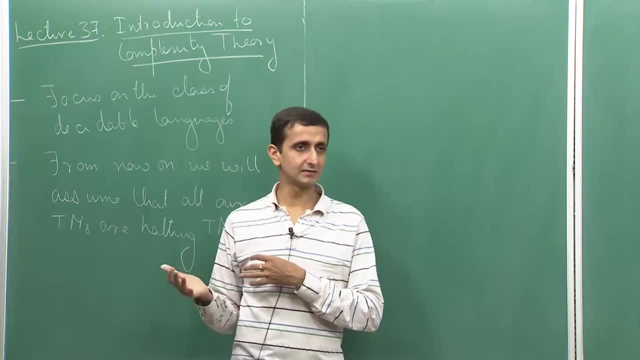 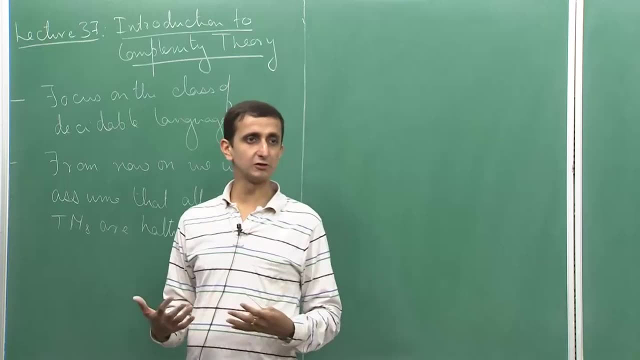 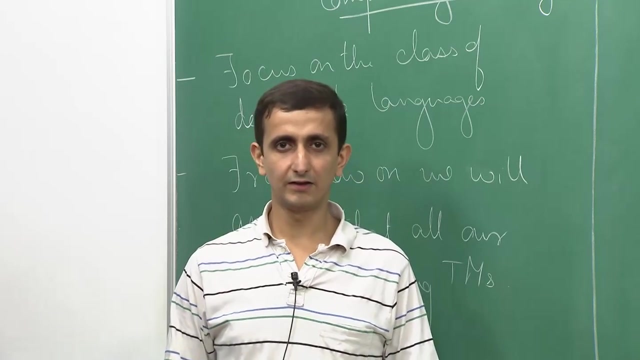 So class of languages which take more time should be in one class, Class of languages which take lesser time should be in another class, and so on. Similarly for resource like space also, we will give a space based on the amount of cells that the Turing machine uses to come up with its answer. 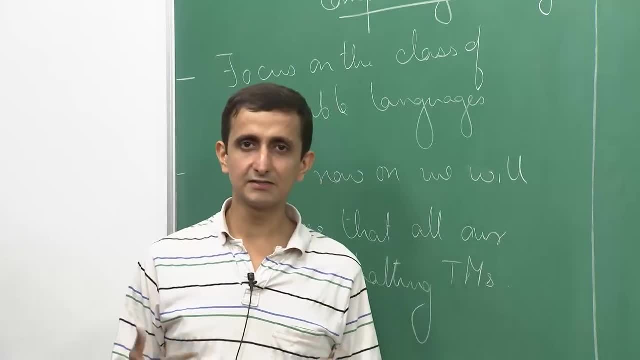 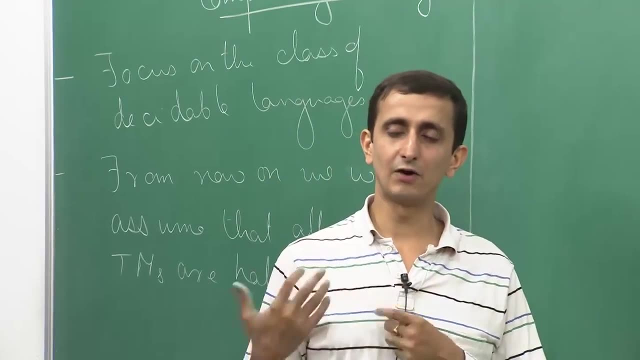 So first, so this gives us classes, and then we will try to, and then we will study relation between these classes. So that is the goal of complexity theory, that how are these classes connected to each other? whether we can show the classes are the same. 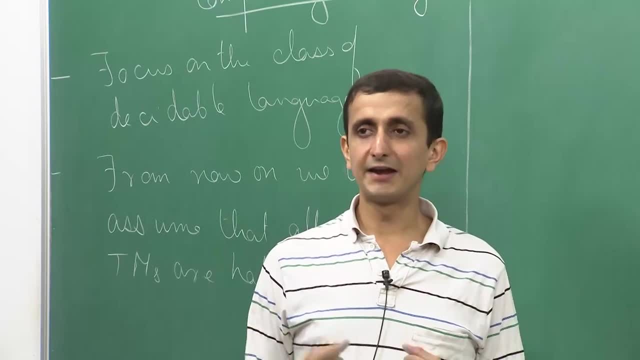 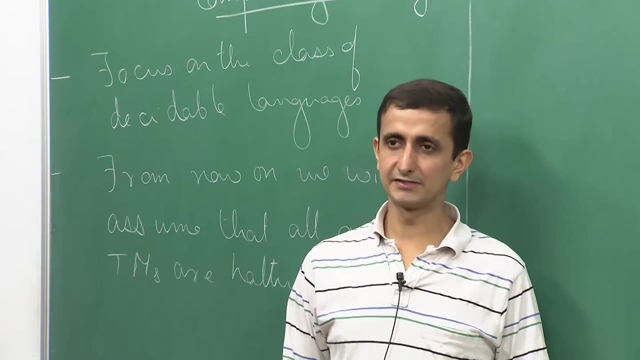 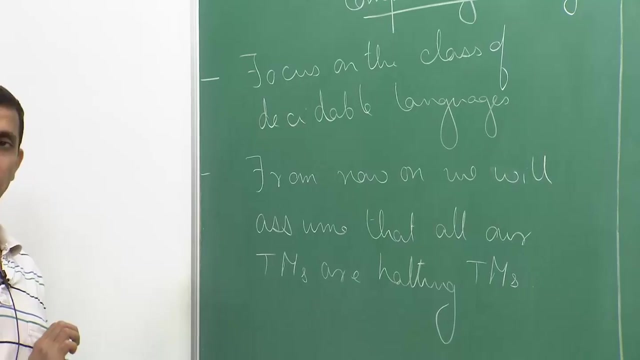 Whether we can separate the classes, What kind of separations are known, and so on. So these are the kind of questions that we try to address in complexity theory. So first we need to define what we mean by running time and space used by a Turing machine. 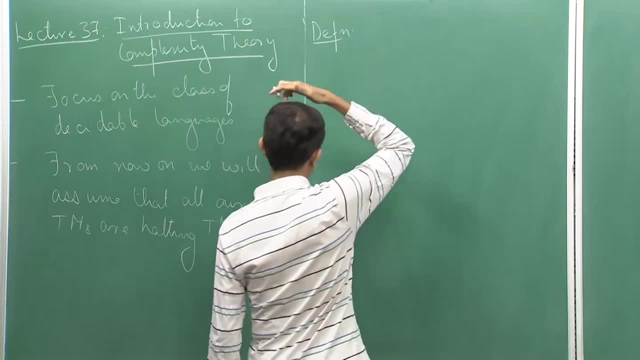 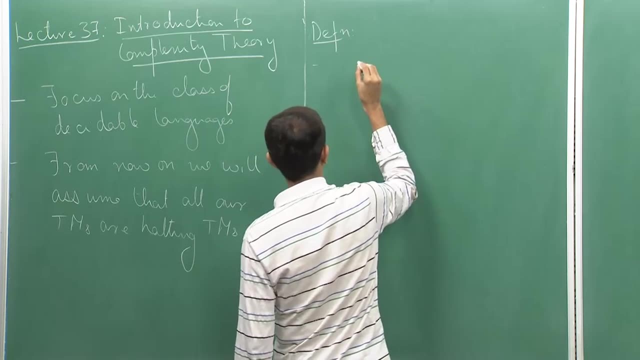 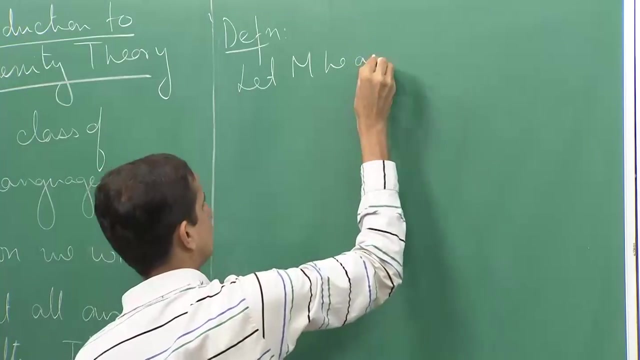 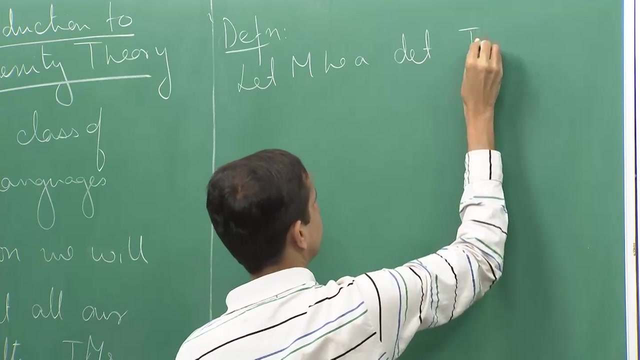 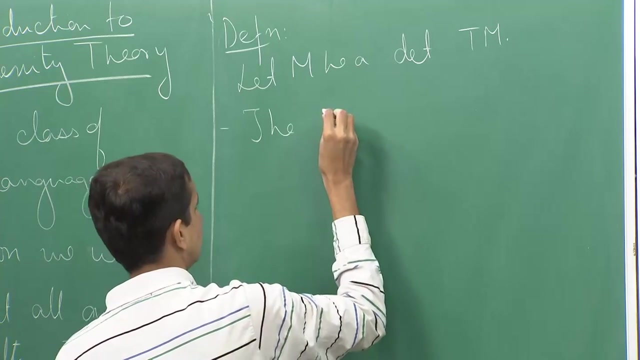 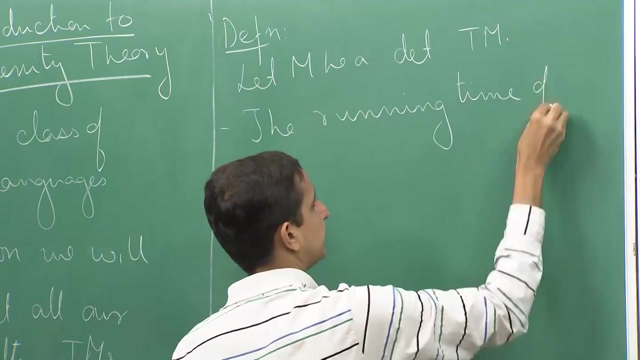 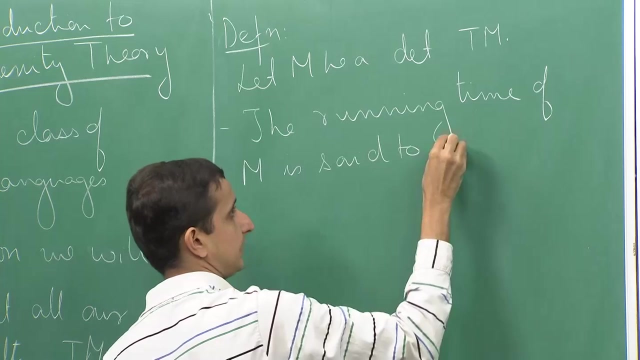 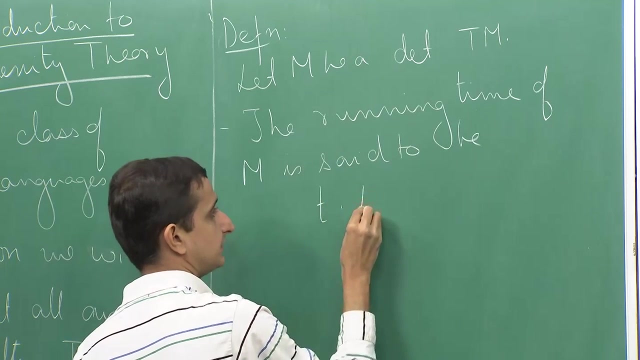 So let us look at few definitions. So first we need to define what we mean by running time and space used by a Turing machine. So let us look at few definitions. So let m be a deterministic Turing machine. The running time of m is said to be t, which is a function from natural numbers to natural 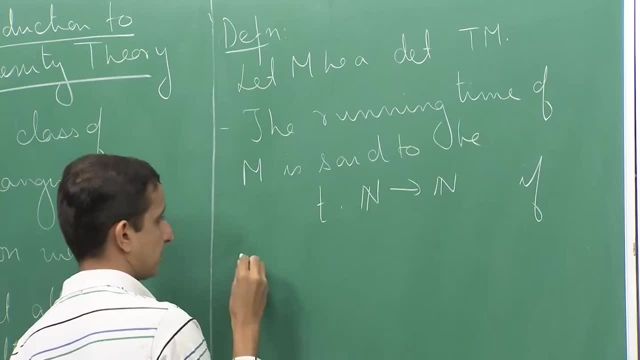 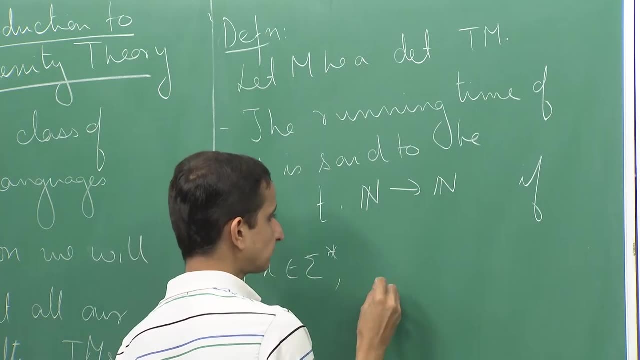 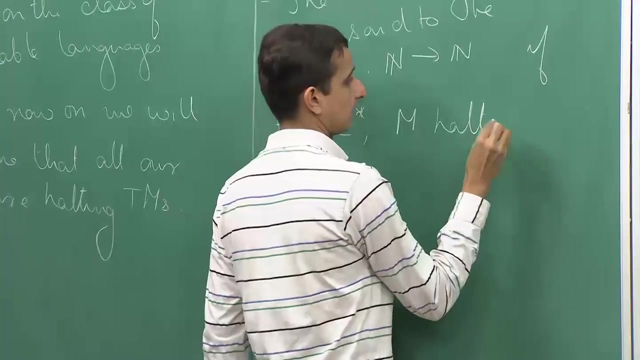 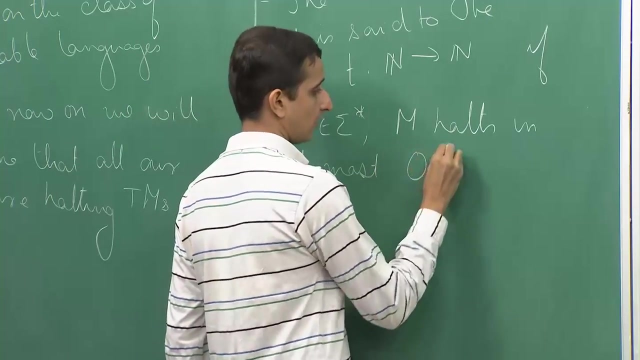 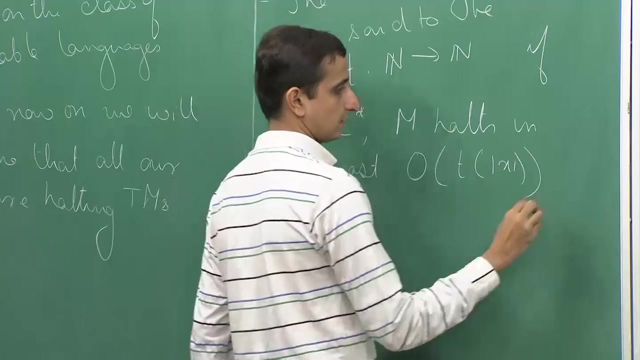 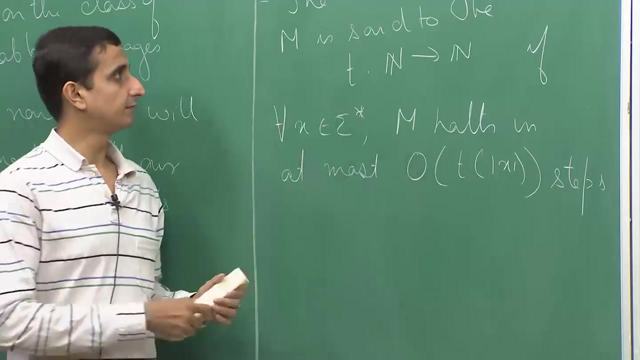 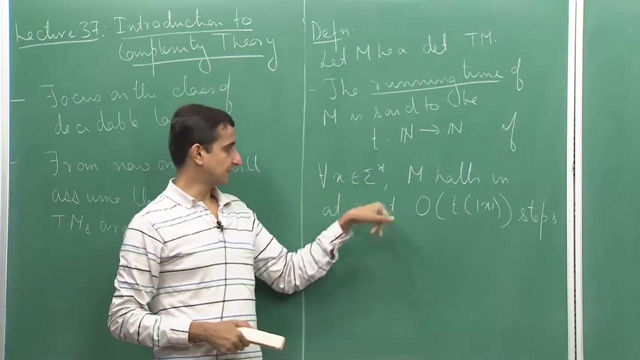 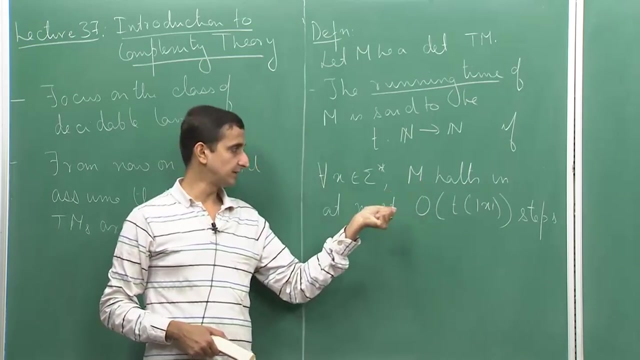 numbers. if for all x in sigma star, so if for all x in sigma star m halts in at most order t of mod x. So we say that the running time of a Turing machine is some function t. if for every x the machine halts in at most order t of mod x steps. So there are several important points. 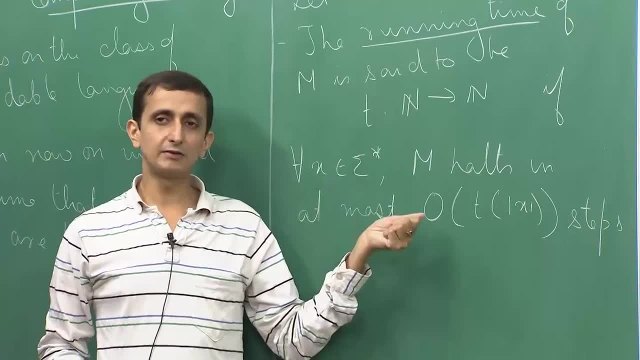 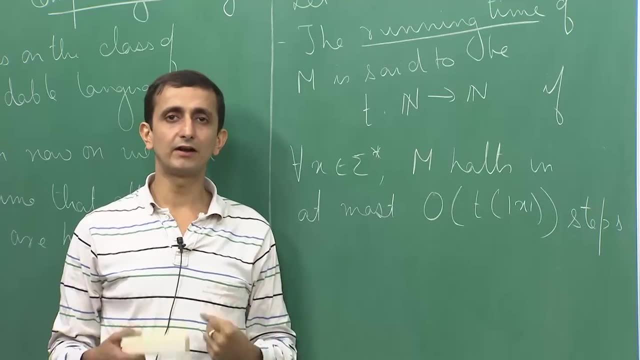 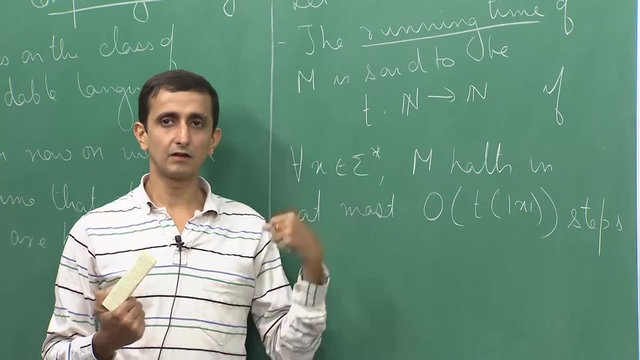 in this definition. First is that we always compute the running time as a function of the length of the input, And not only for running time. even when we look at other resources, such as space, the amount of resource that is used by a Turing machine is always a function. 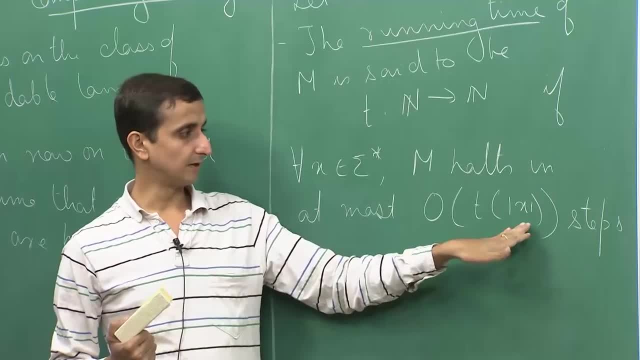 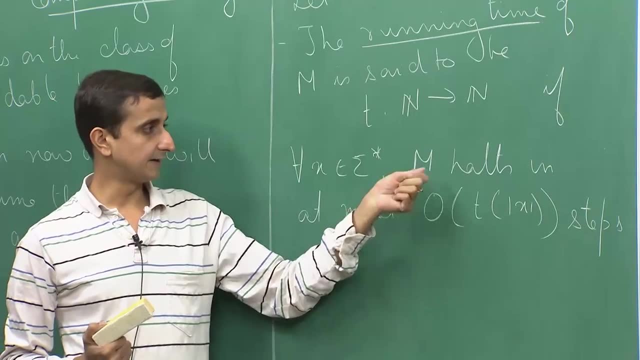 of the length of the input. So if x is my input, it is a function of the length. Next, is that? so here we talk about the running time. So we say that the running time is t if on input x, the machine m. 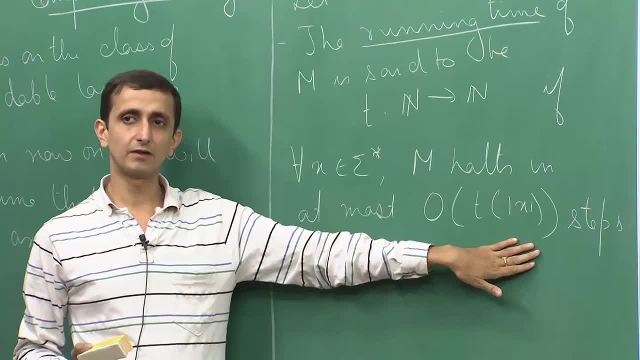 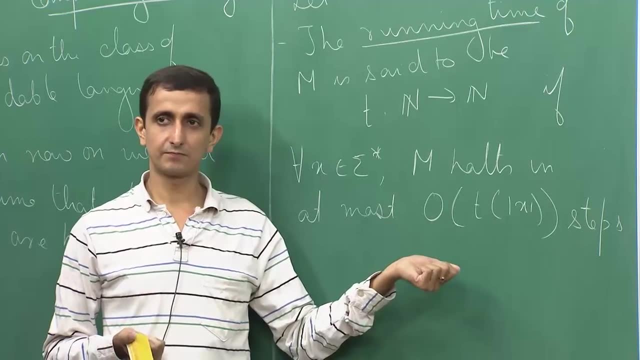 And t is just a function of each variable that is required to run time in order. t is just m, which we can say as m average. If Turing machine h is a function of the width of the information when m is in this books, which is Poisson's equation, Such that it 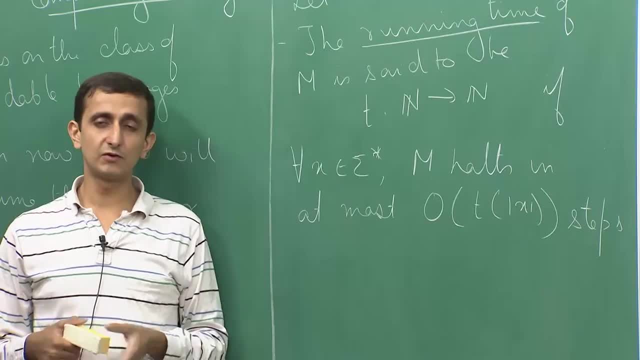 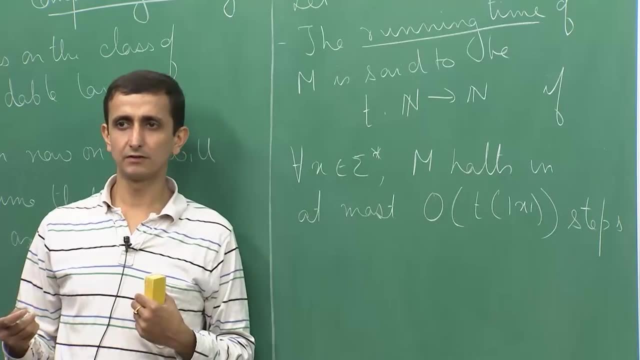 would be round. x is the quantity of the additional flow on this economy. Now what we will be doing is to calculate. v is at x square. If Turing machine is having a feed value of t, it is taken rather by a term like this: plus, there are time constraints If t is on that. 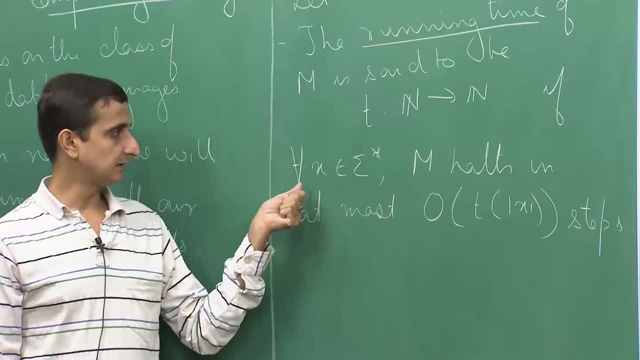 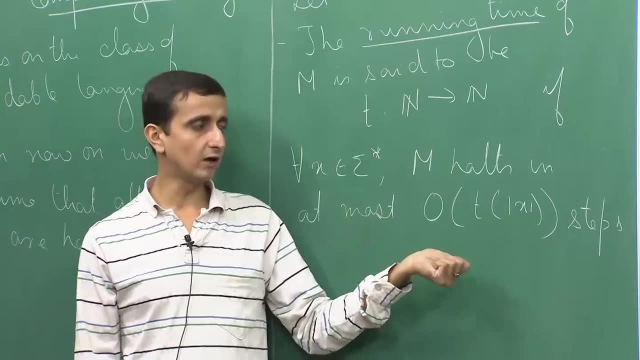 point, let us say about this problem of condition. then also it has got to be an origin function. maps n to n square. then we say that the machine has running time n square if for every x the machine holds in at most order n square number of steps, So it can take for example n square. 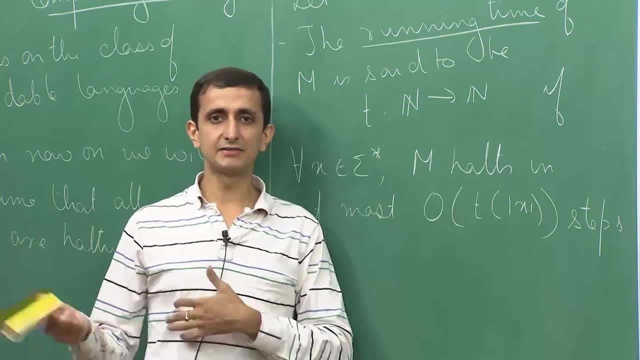 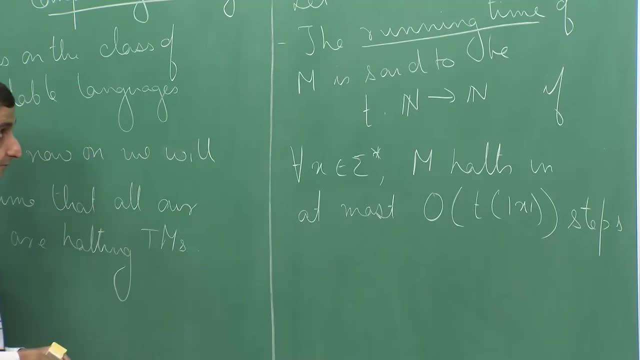 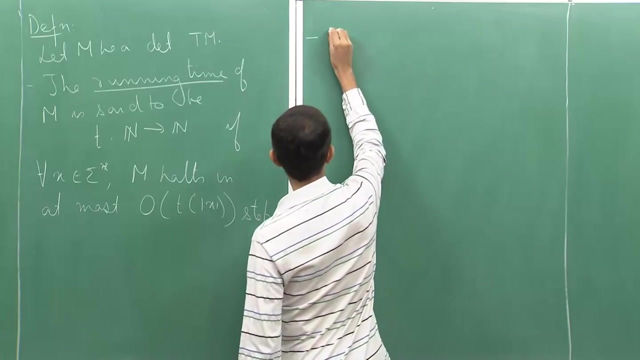 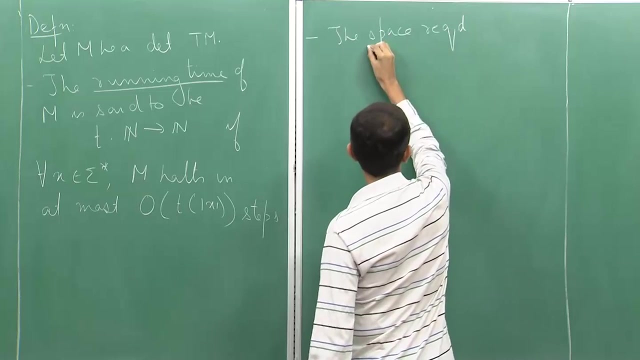 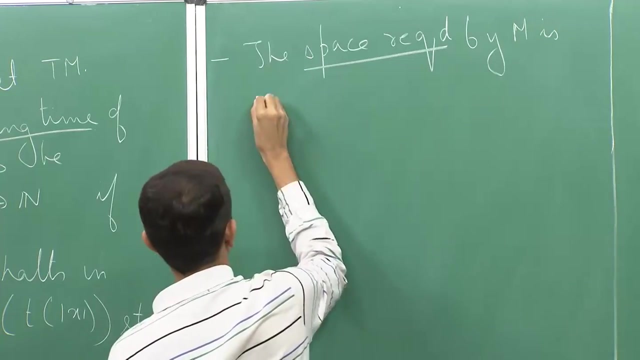 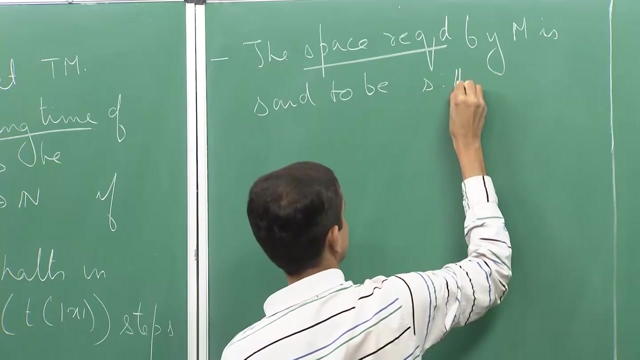 plus n, or 100 n square minus 2, n plus 3 or any such thing which belongs to the class order n square. So, similarly, we define the space required by M is said to be the function s going from to n. So we define this as the space required by M is said to be the function s going from. 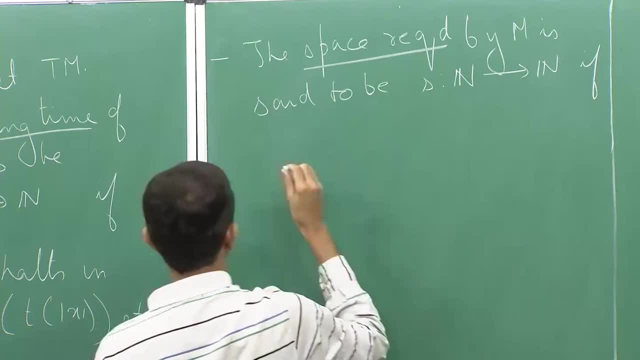 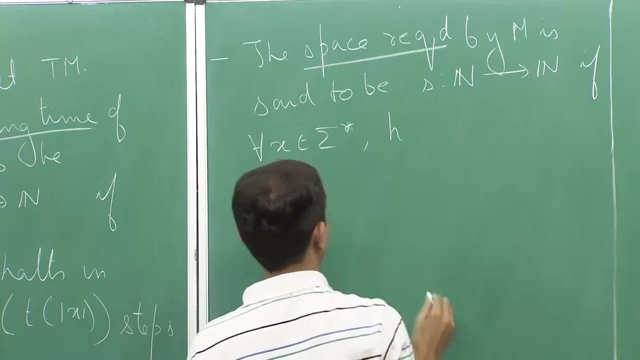 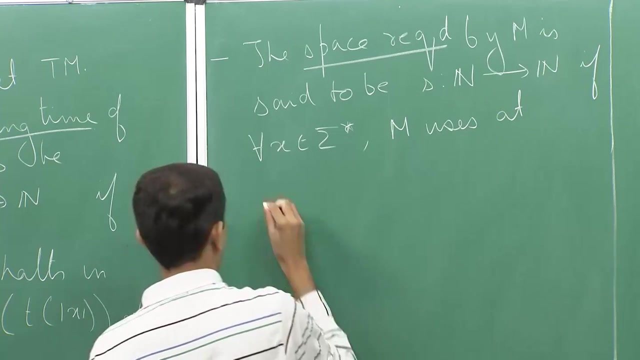 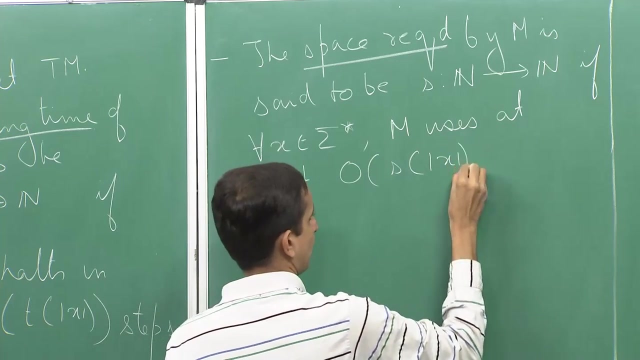 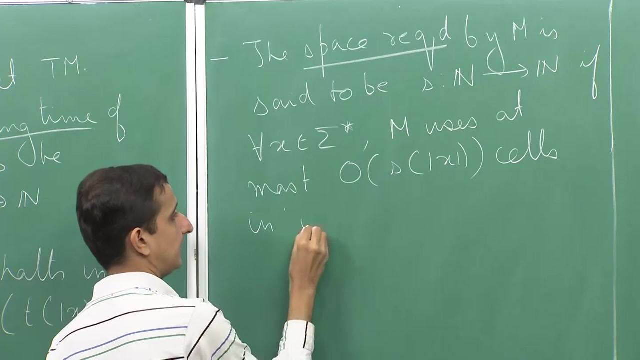 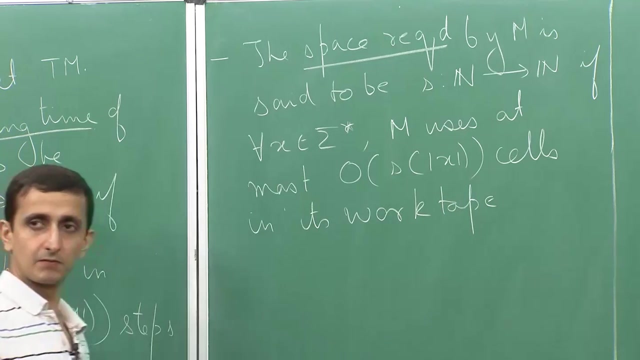 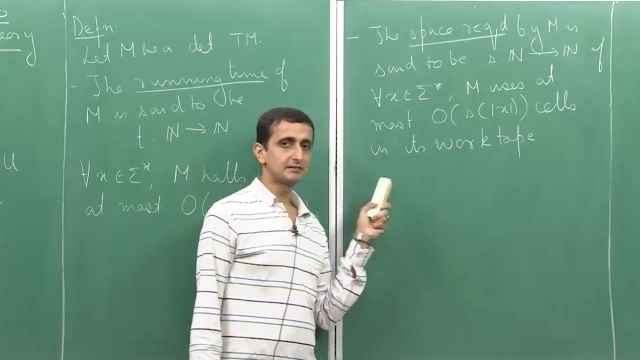 n to n. if for all x in sigma star M uses at most order S of mod x cells, at most order n is in its work tape. So one additional point that is important here is that when we are looking at space complexity it is important that we keep in mind the model that 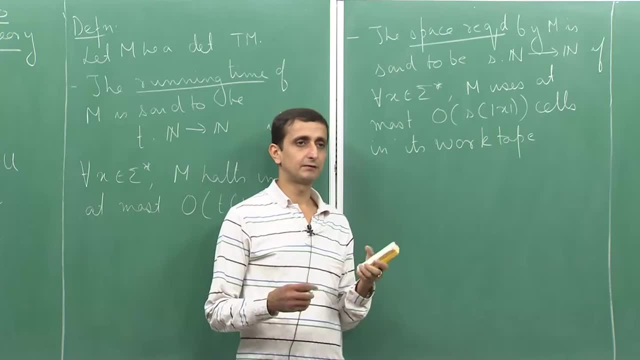 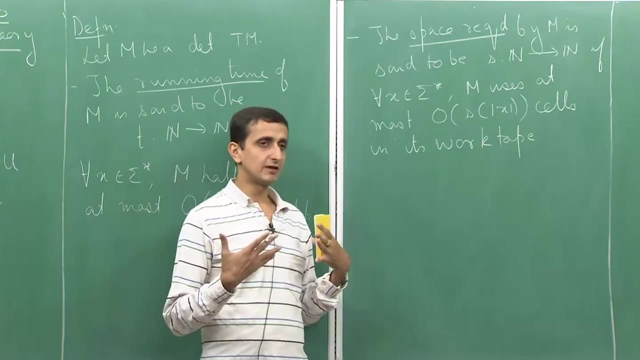 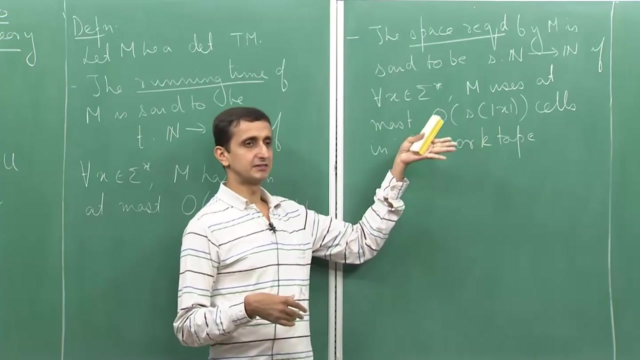 we defined or we discussed last time. So we have a Turing machine- not last time when we talked about reduction- Turing machine which has 3 tapes: input tape, work tape and output tape. So when we talk about space complexity of a machine, we do not consider the space used in the input tape. 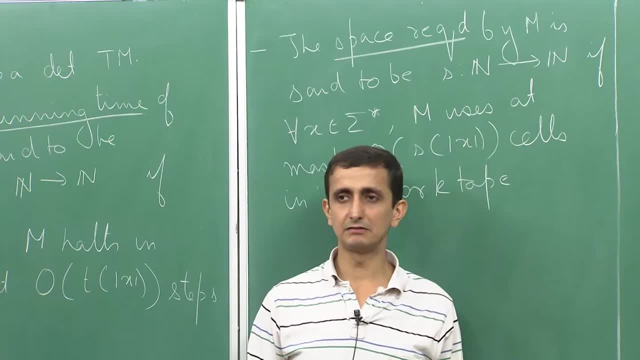 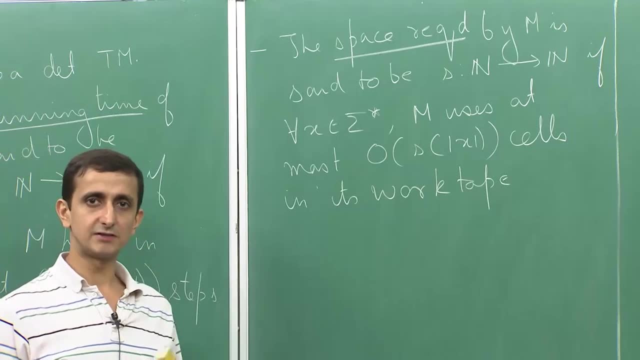 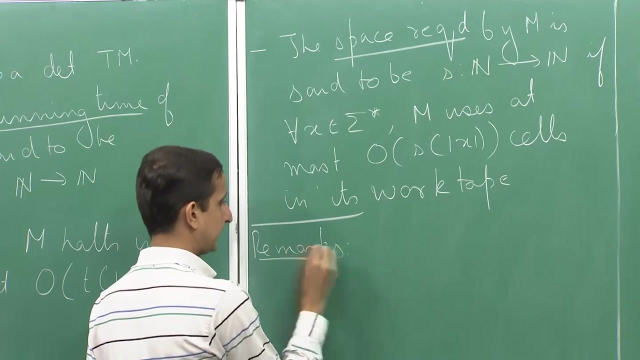 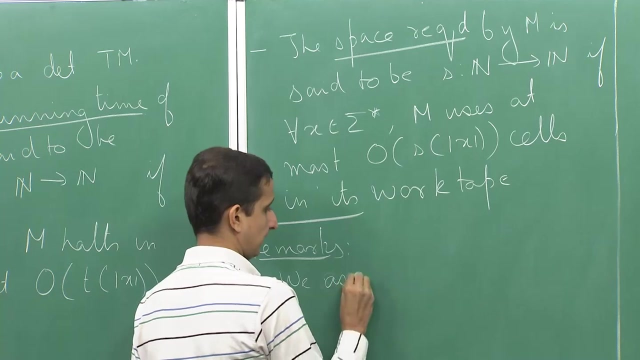 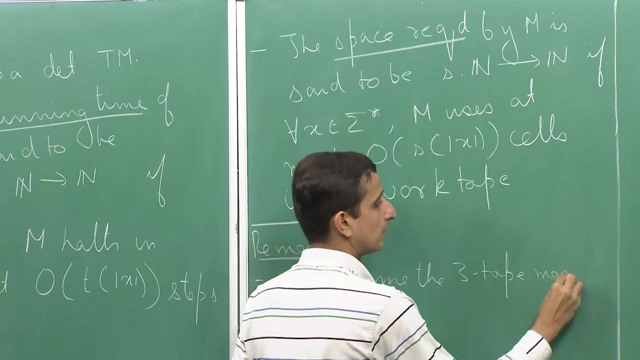 and the output tape. So they can be anything, that is any arbitrary amount. We only look at the space used in the work tape of the Turing machine, the amount of cells used in the work tape. So remarks, So let me quickly mention what I said. So we assume the 3-tape. 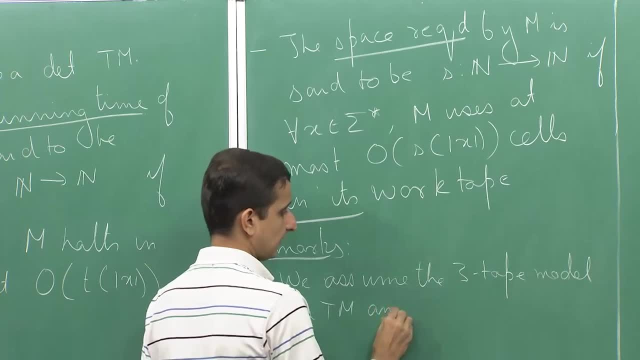 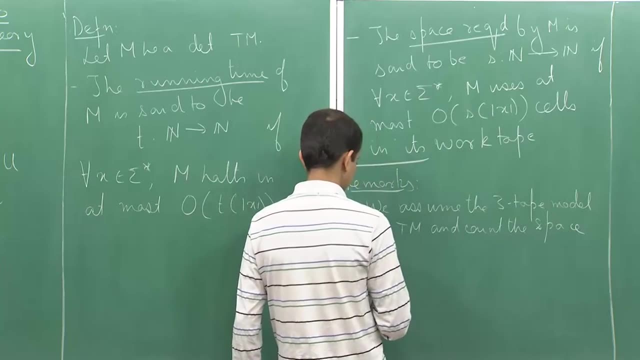 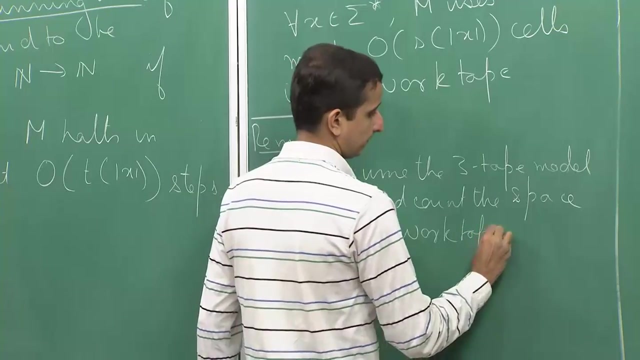 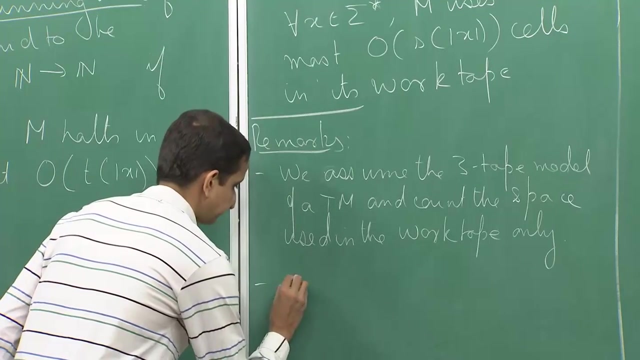 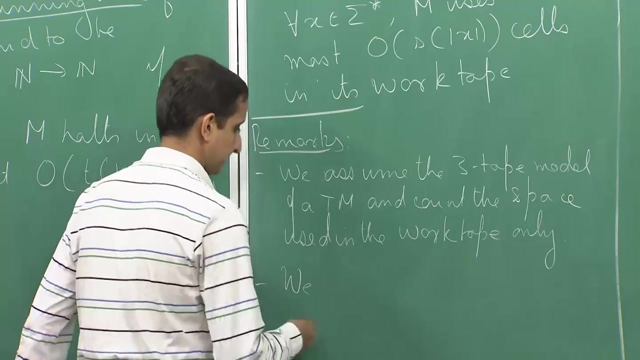 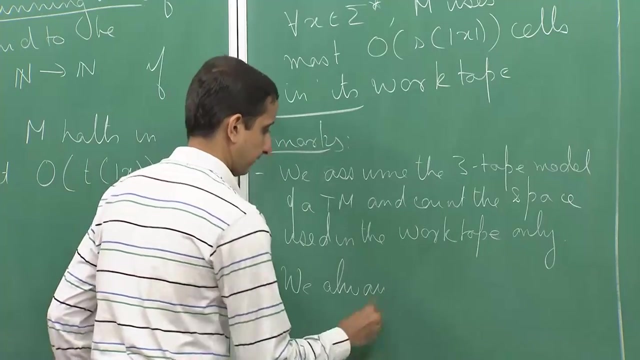 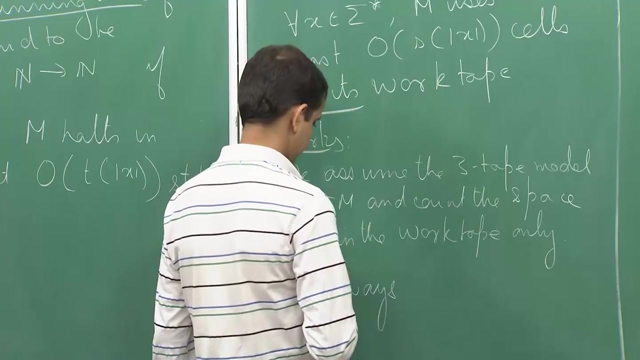 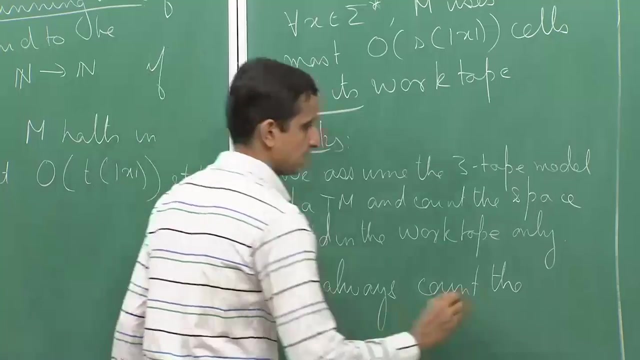 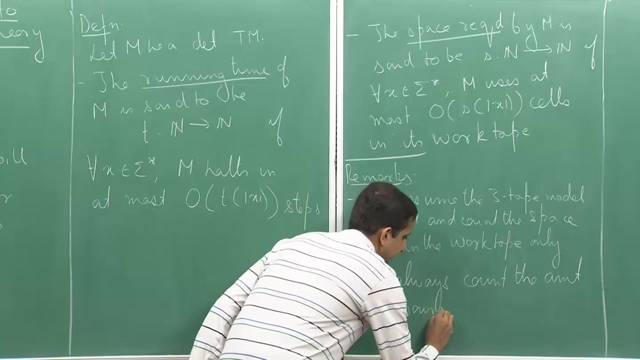 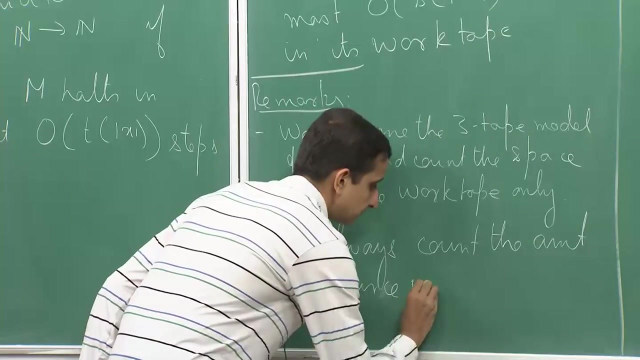 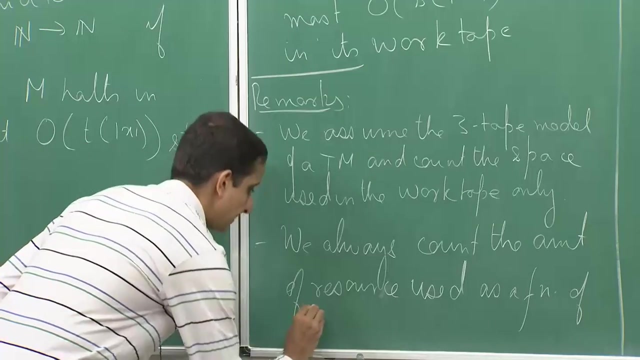 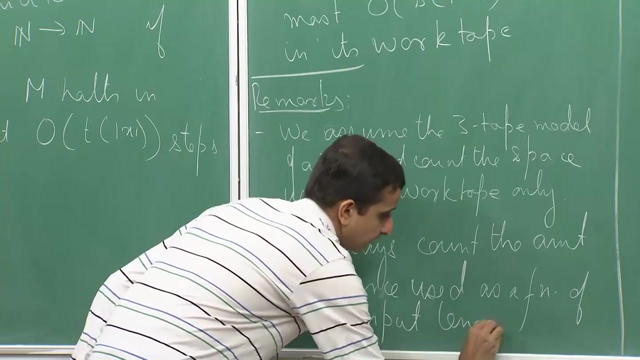 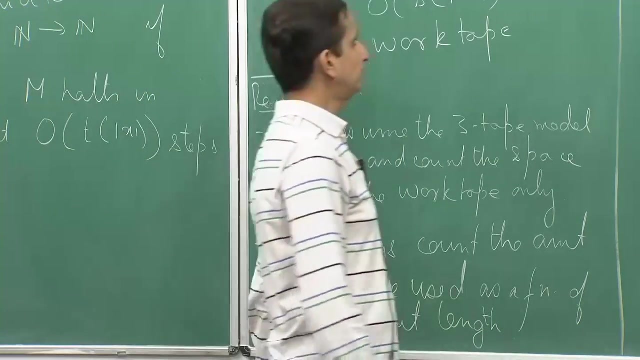 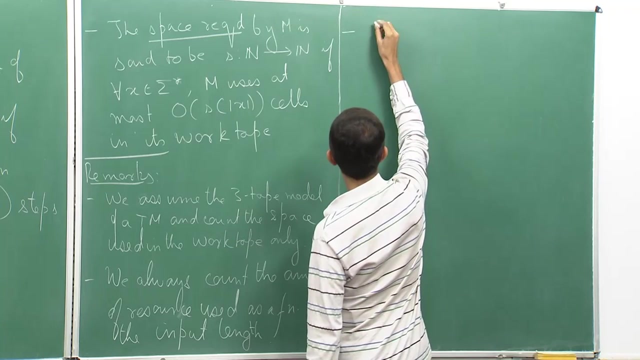 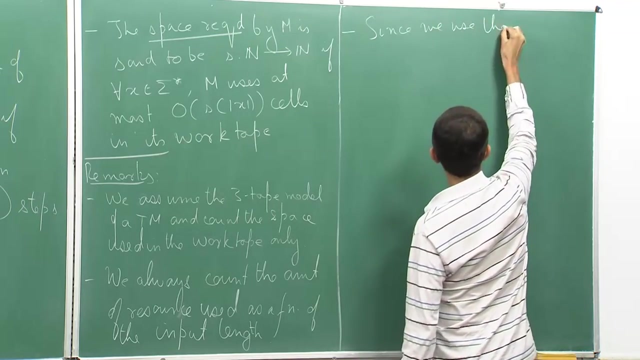 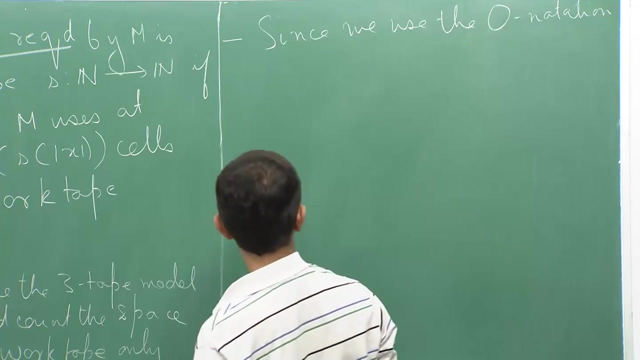 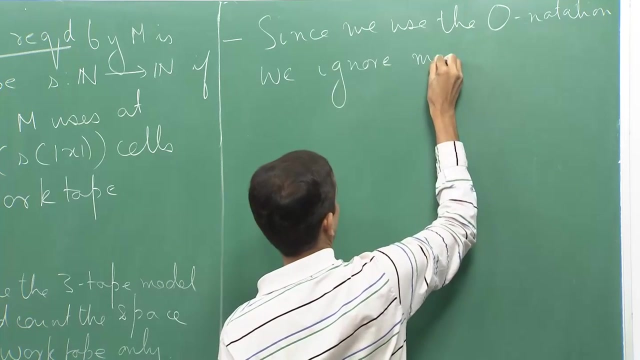 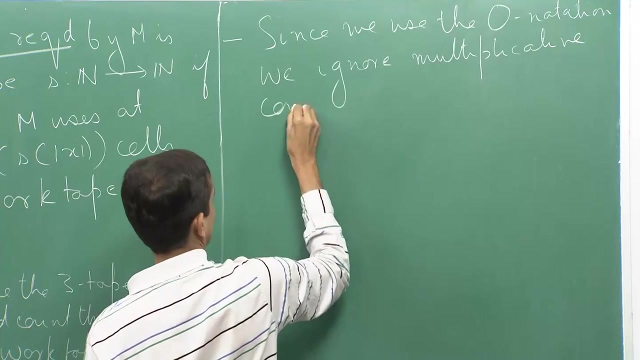 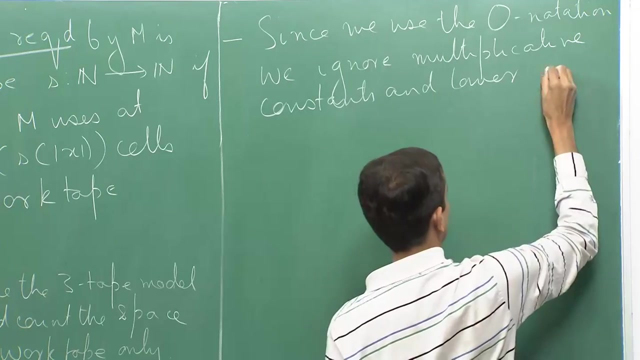 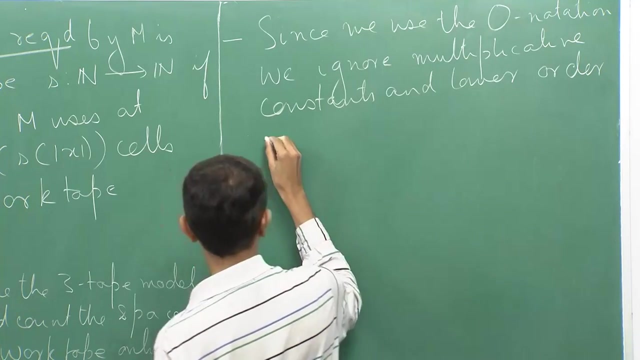 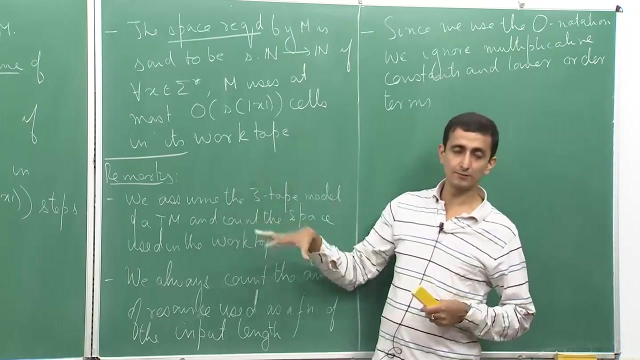 model of a Turing machine and count the total number of cells used in the Turing machine. So this is the space used in the work tape only. Second, is we always? So, now that we have defined time and space complexity, or we have defined what we mean? 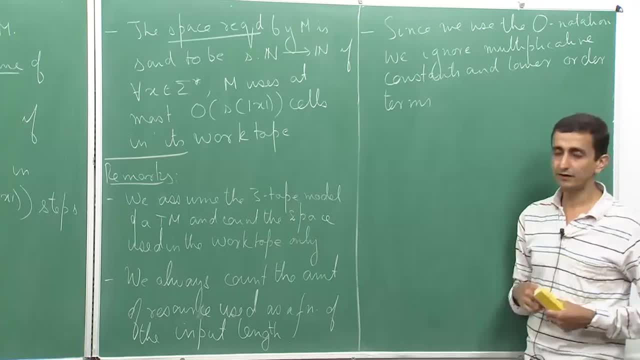 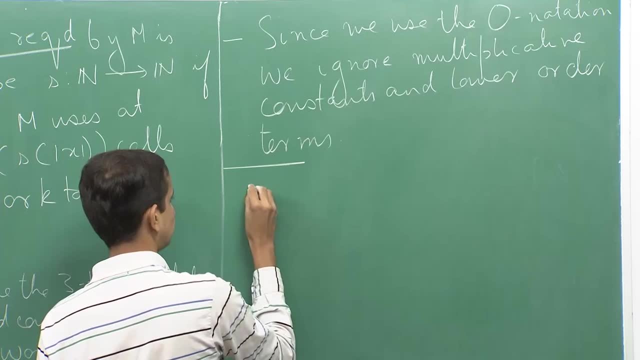 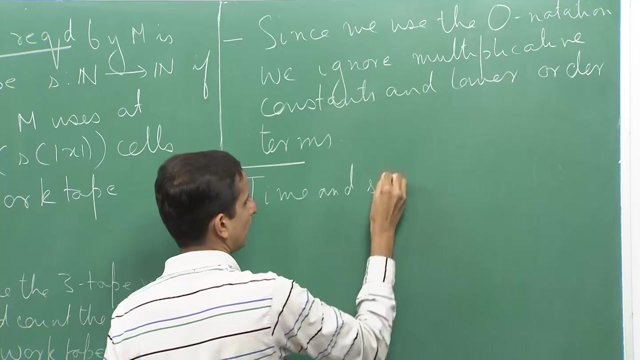 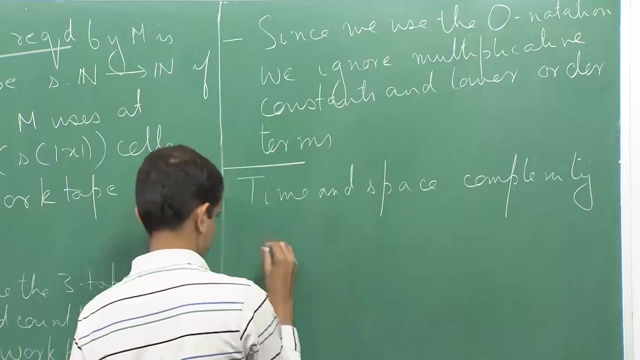 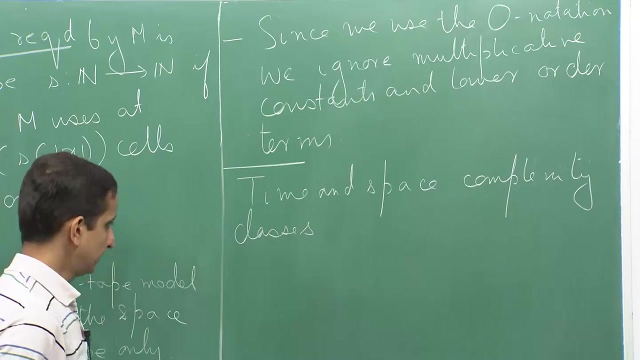 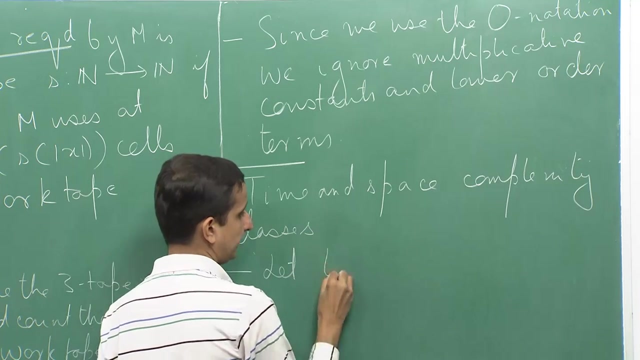 by running time of a machine and the space used by a machine, we can define the time and space complexity classes. So let be a function from natural numbers to natural numbers. So this is the time function that 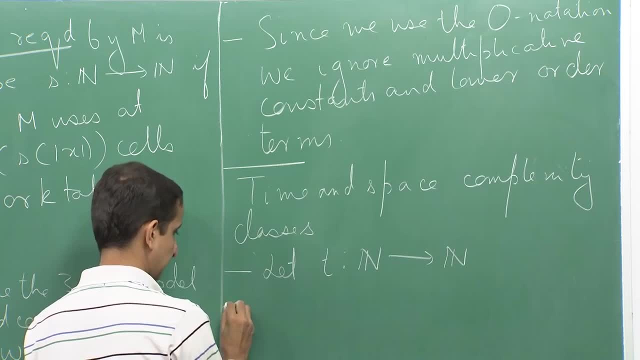 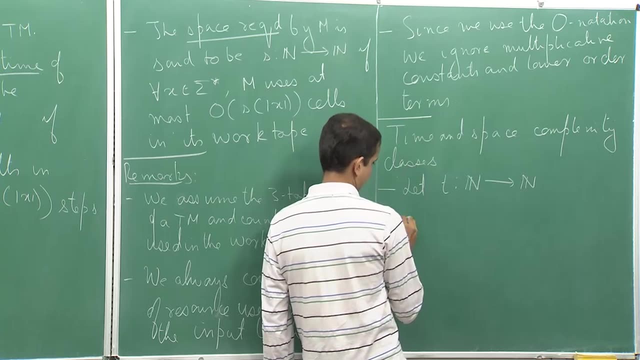 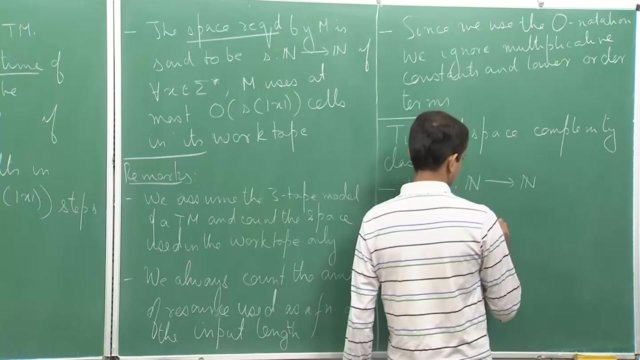 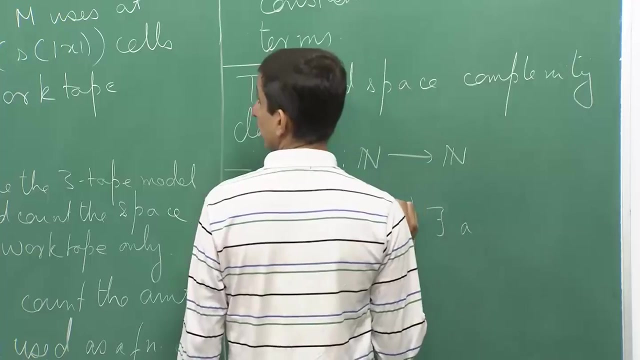 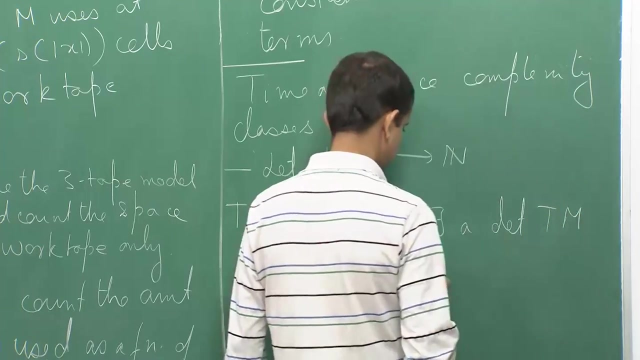 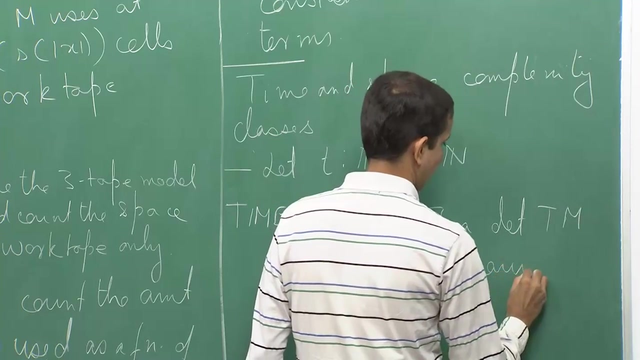 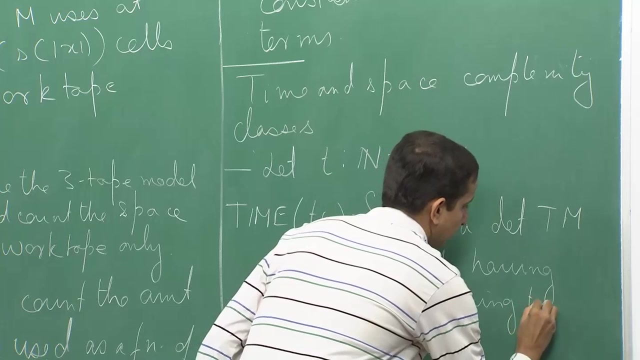 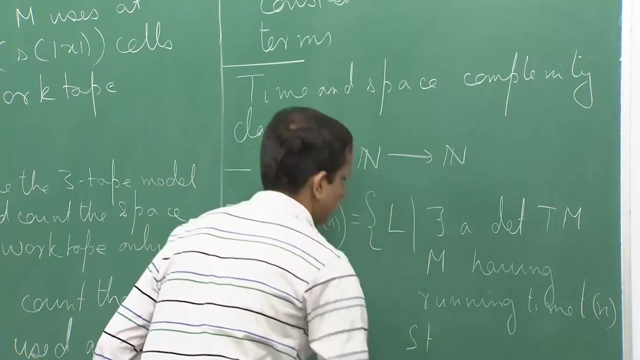 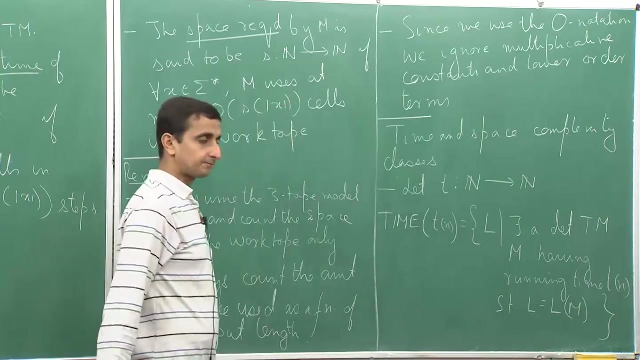 we will have. We define the class d, time t, or we will just call it as time t, time t of n, as the class of languages, l such that there exists a deterministic Turing machine, m having t of t running time t of n such that l equals l of m, So time t of n consists of all languages. 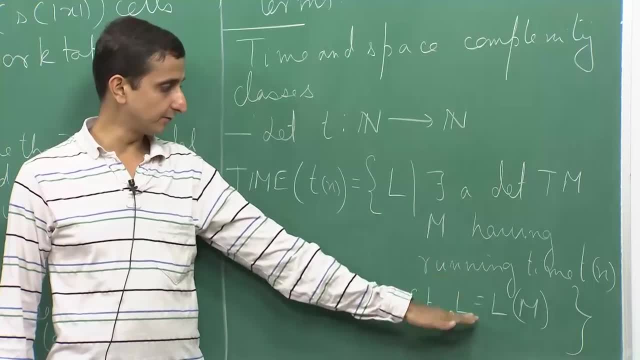 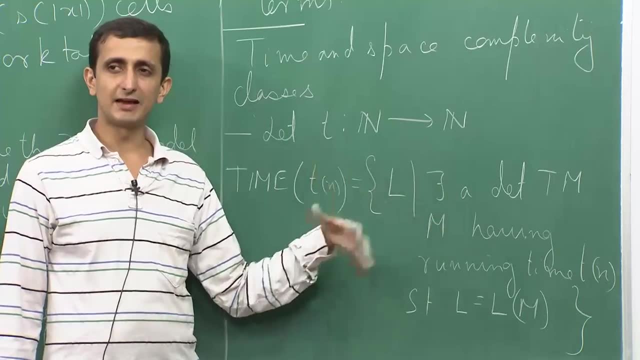 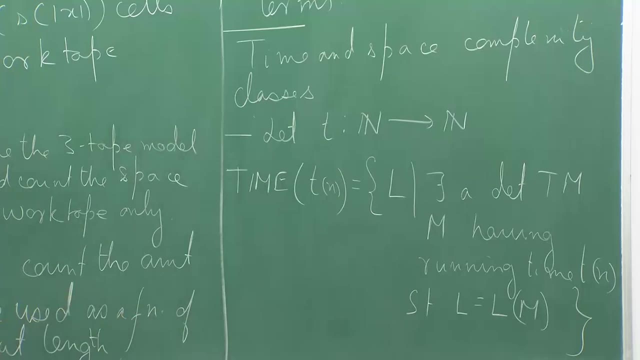 for which there is some Turing machine that has running time t of n and it accepts the language l. So basically all languages for which we have some algorithm or some program which runs in that many number of steps. So that is the idea. 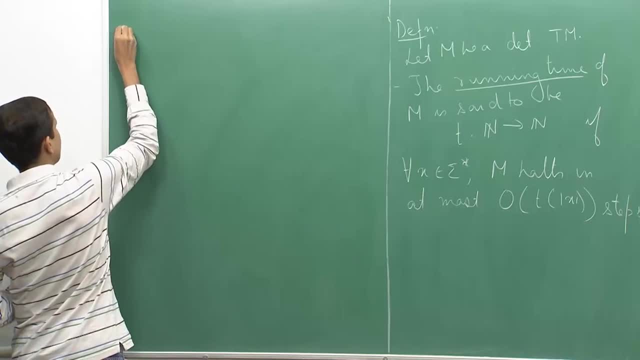 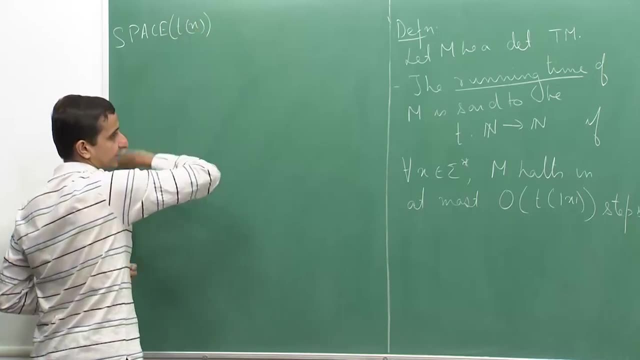 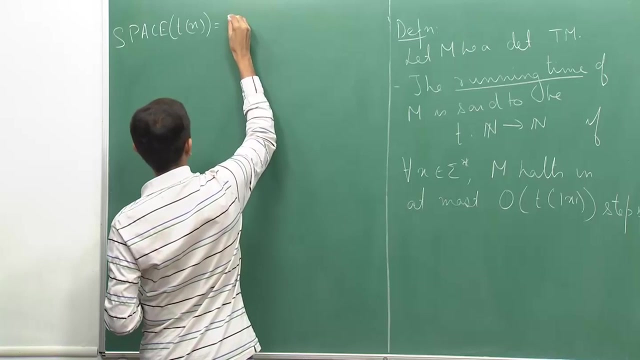 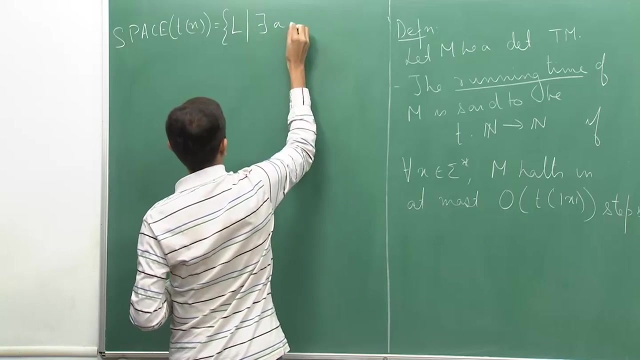 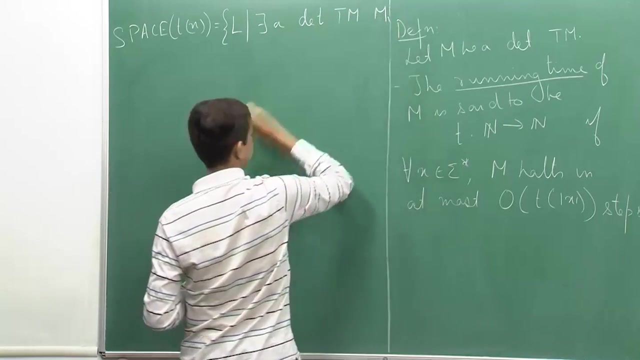 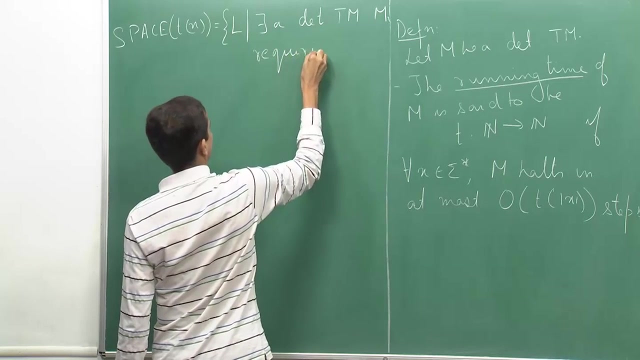 Similarly for space also, we define space t of n as t of n. The class of language is l, such that there exists a deterministic Turing machine, m, requiring a t of n. So t of n is a deterministic Turing machine. So t of n is a deterministic Turing machine. So t of n is a deterministic Turing machine. 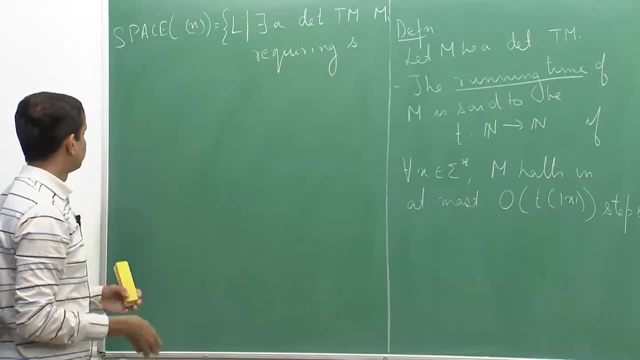 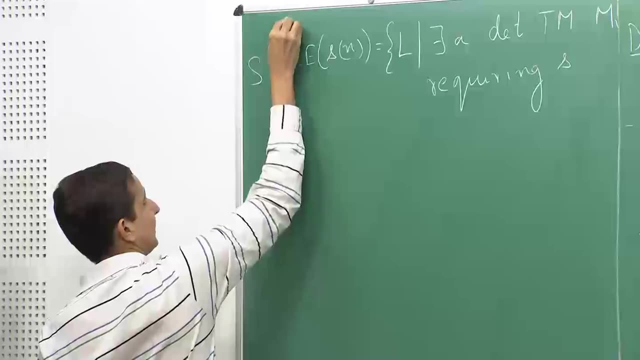 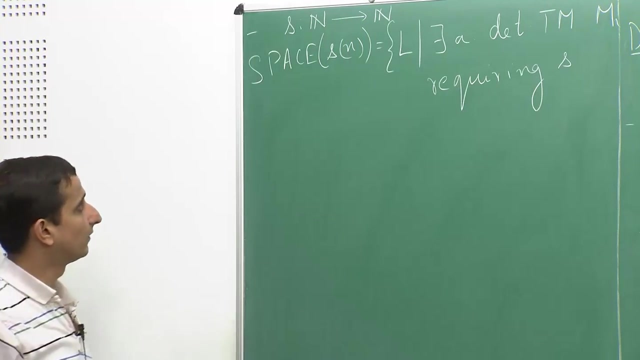 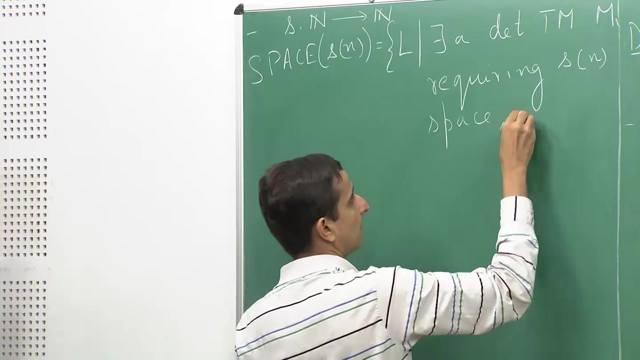 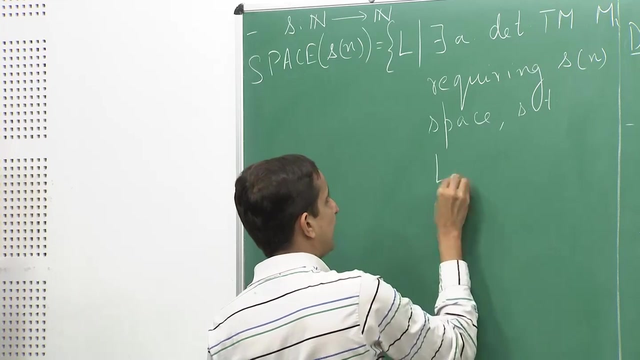 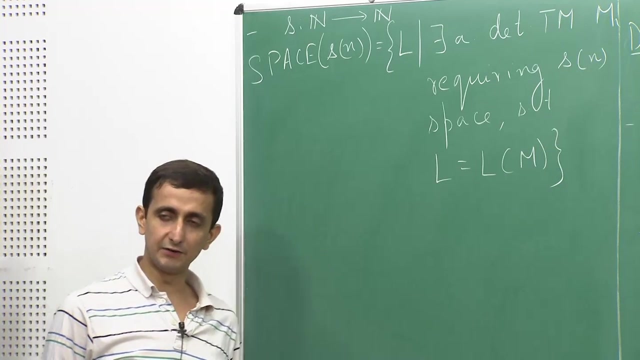 So for space, let me use, just for more clarity, let me use, the function small s of n. Once again, uh s is a function from natural numbers to natural numbers, so requiring s of n space, such that that L equals L of n. So all those languages for which there is a Turing machine that takes 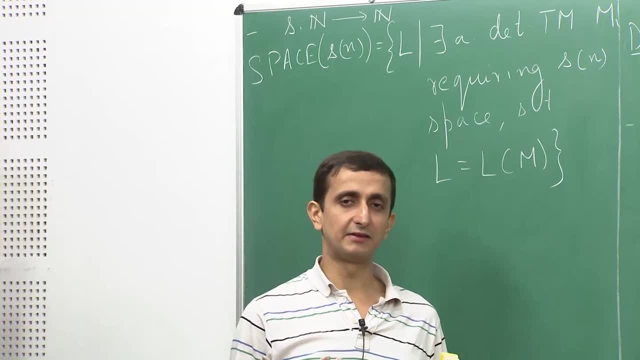 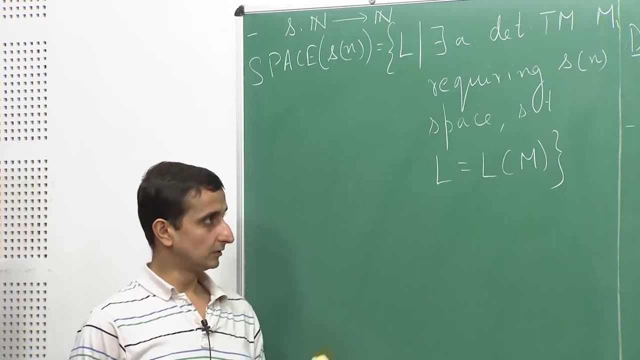 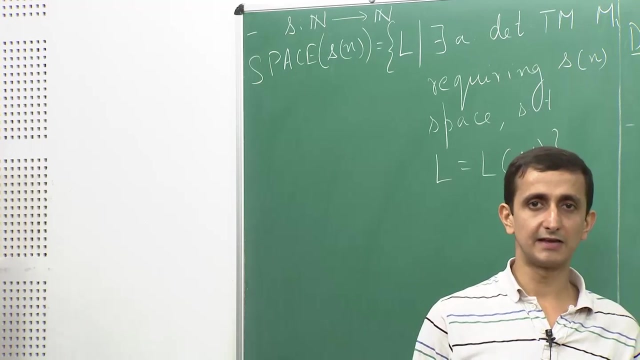 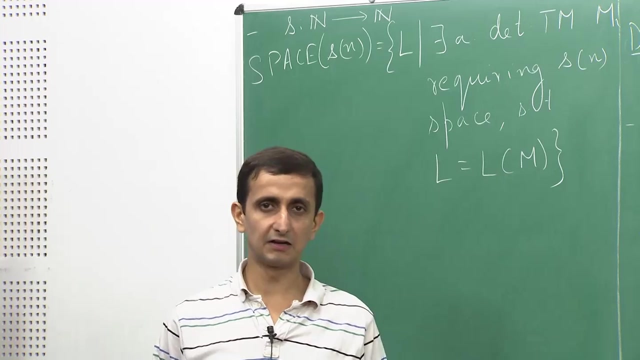 order I mean that uses at most order s of n number of cells or that runs in space s of n. So this is how we define the class time Tn and the class space s of n. So in some texts you will also find them defined as D time and the class D space, but essentially they. 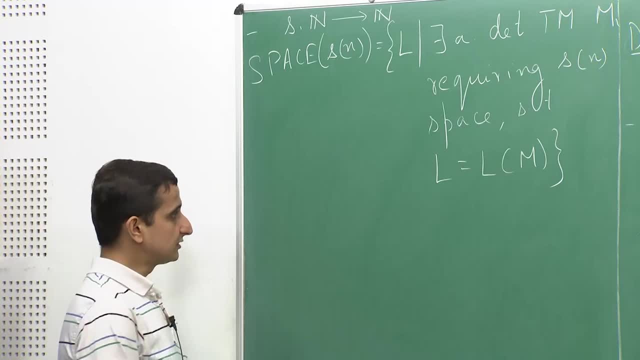 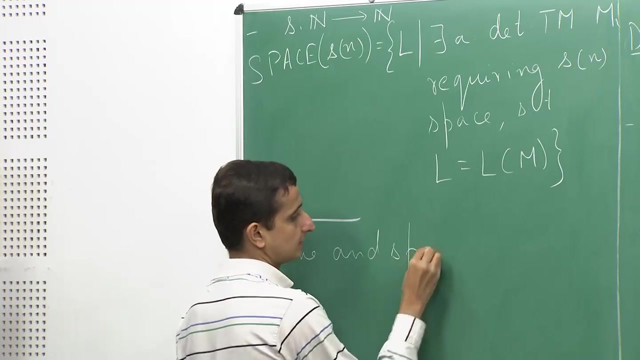 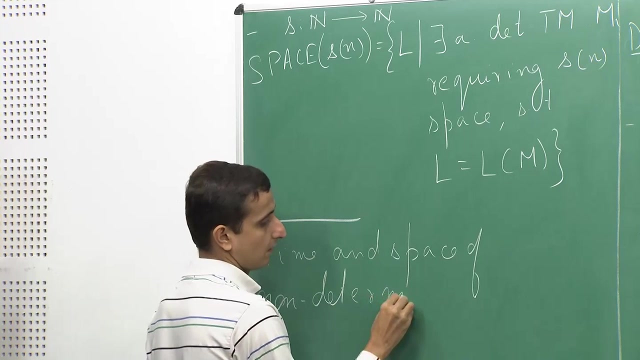 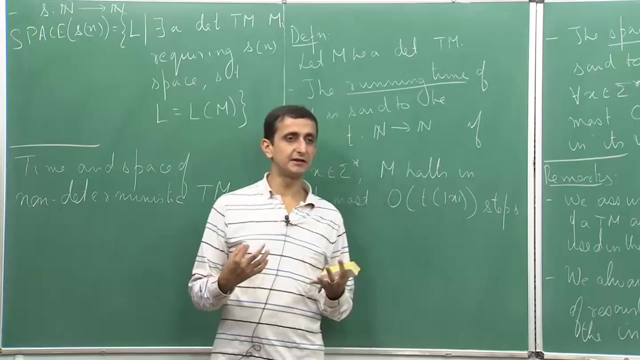 are the same, So now we can also define. so all these was for deterministic Turing machine, So we can also look at the time and space of non-deterministic Turing machines. So in the case of non-deterministic Turing machines we just have to make a call. So how does a non-deterministic Turing behave? 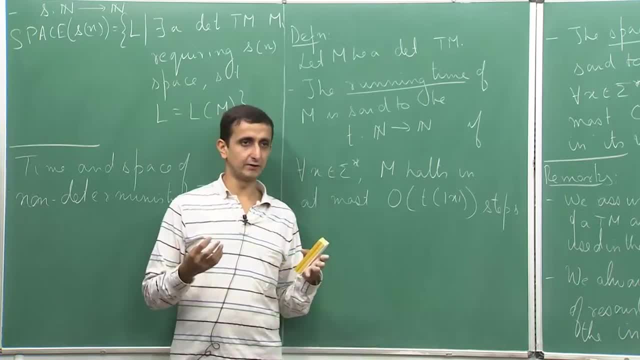 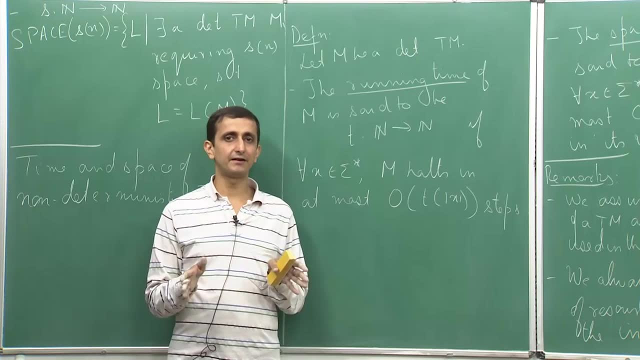 Turing machine behave. So recall that in a non-deterministic Turing machine the Turing machine can non-deterministically branch off at every step. So at every step during its computation it can non-deterministically decide to do maybe one of two different things. 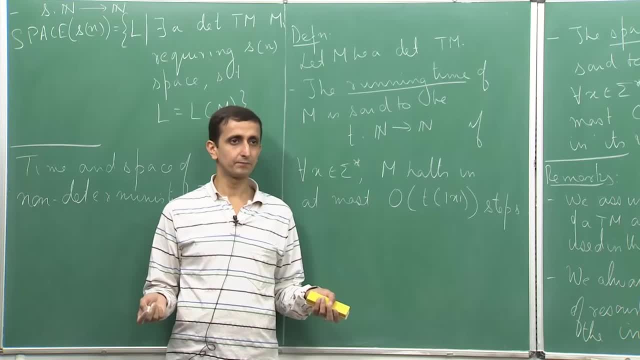 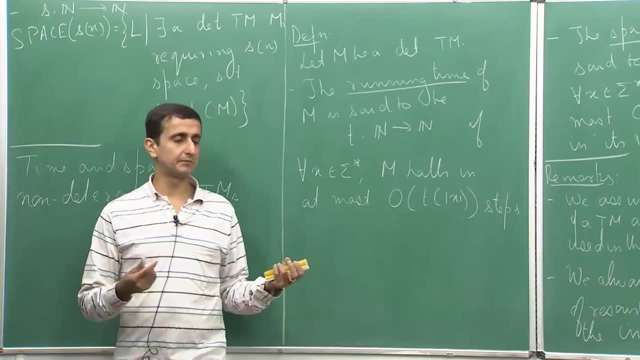 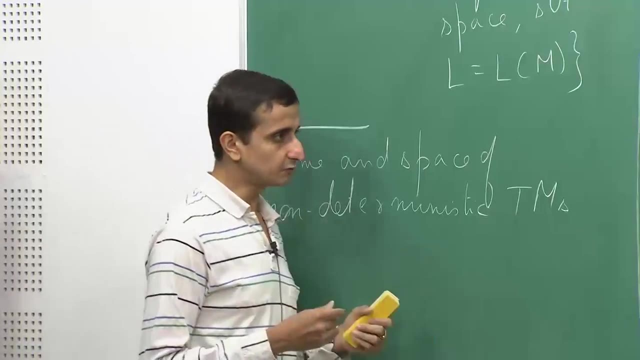 So therefore it will have more than one computation paths that will lead to a accept or a reject state And therefore, when we talk about the running time and the space required, we have to be little careful. So the way we define the running time of a non-deterministic Turing machine is: we look 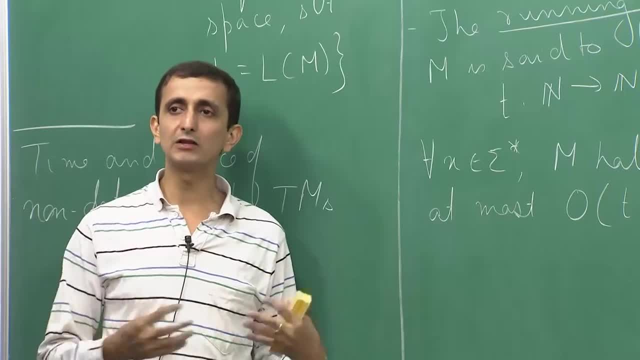 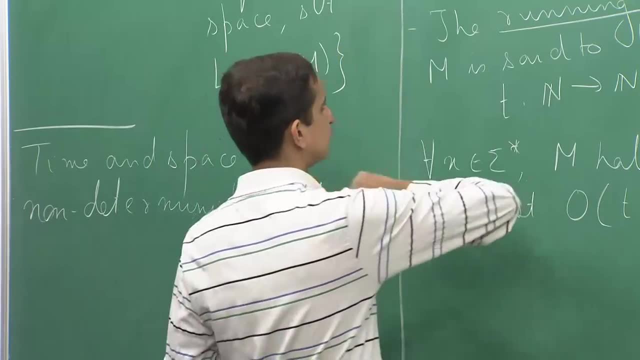 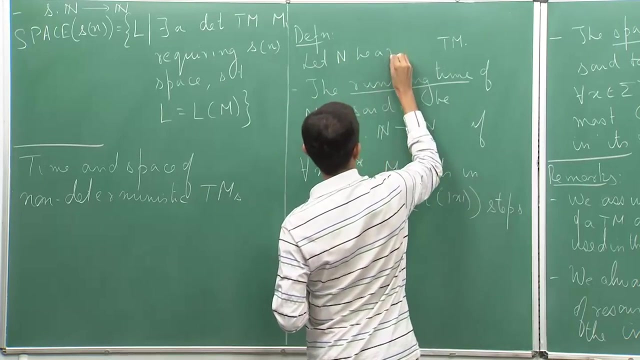 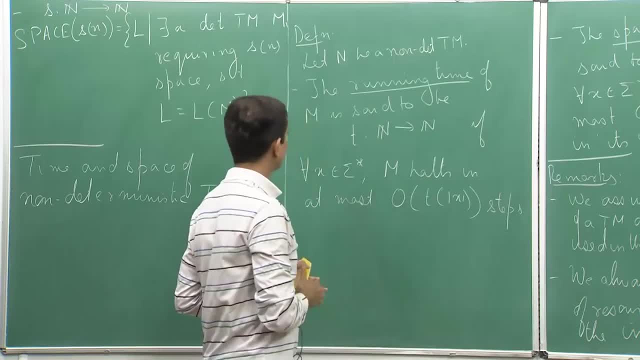 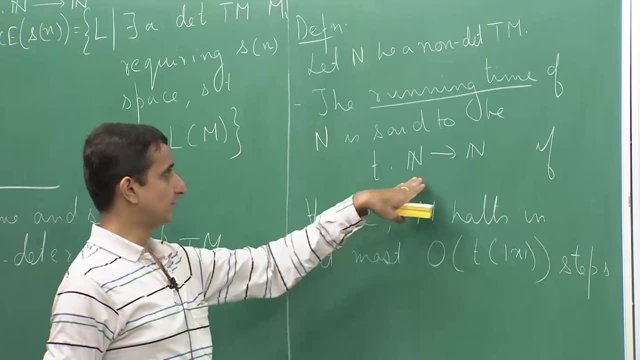 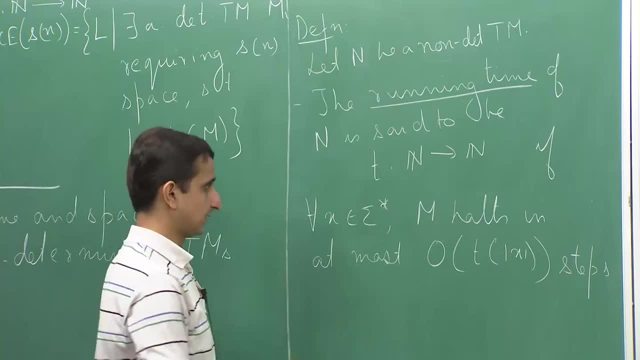 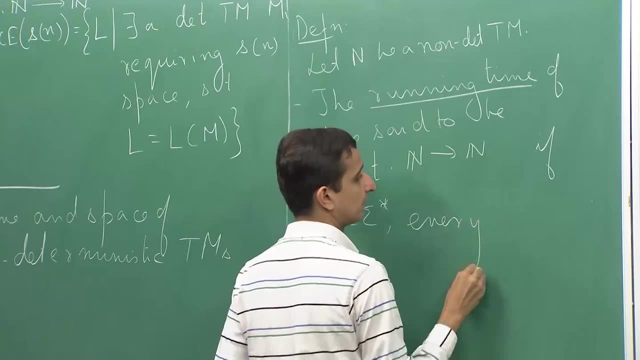 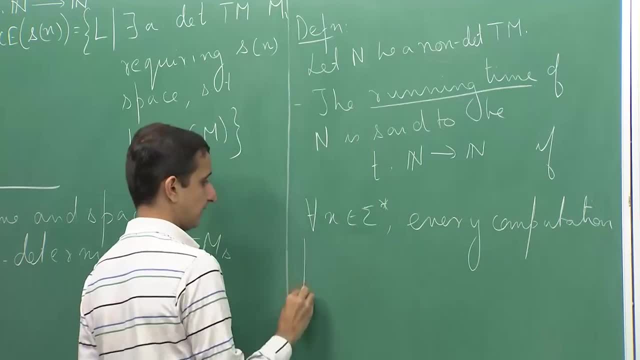 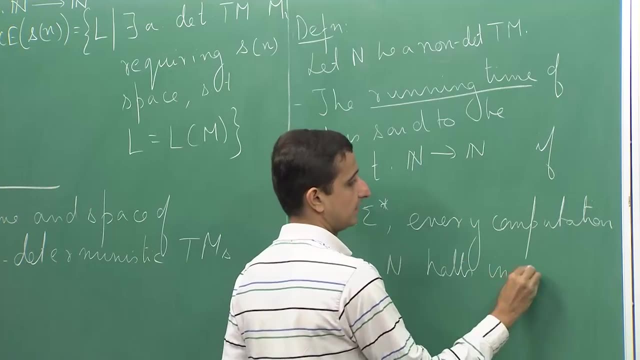 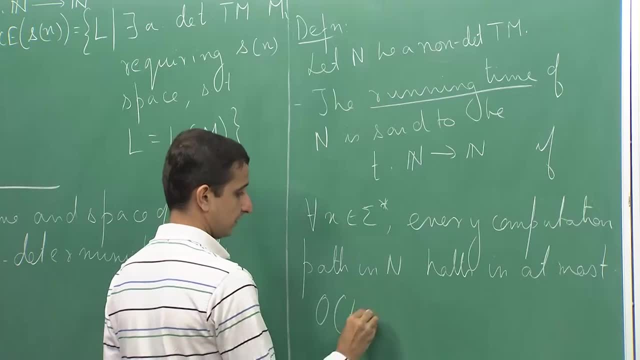 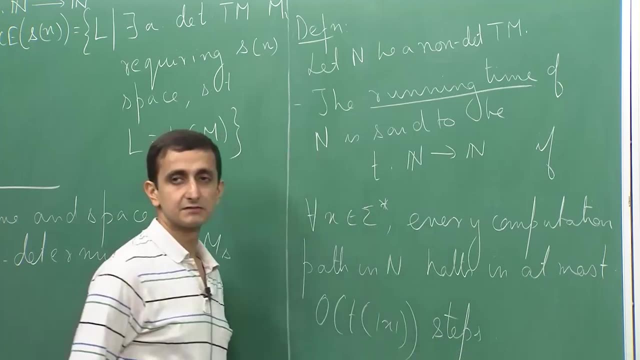 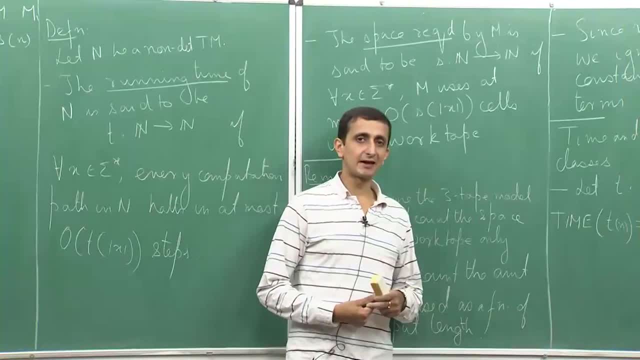 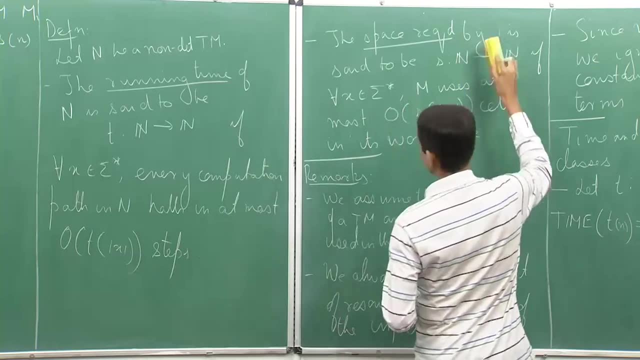 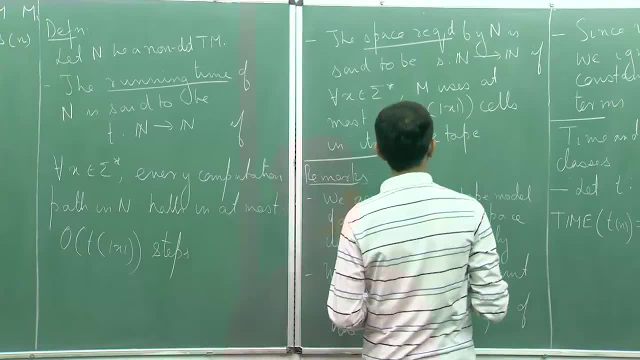 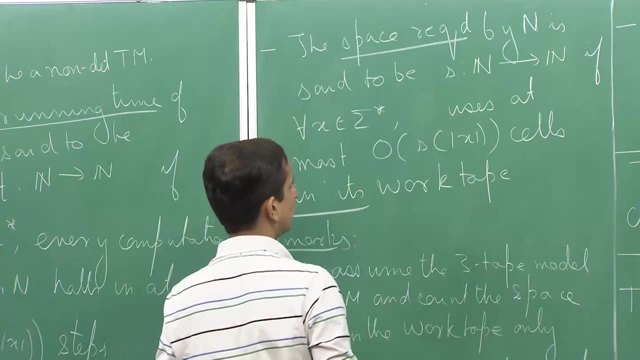 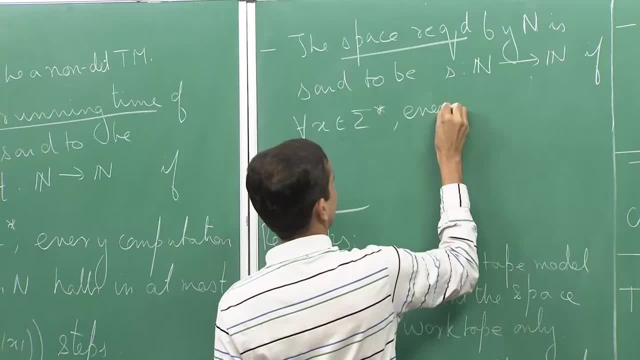 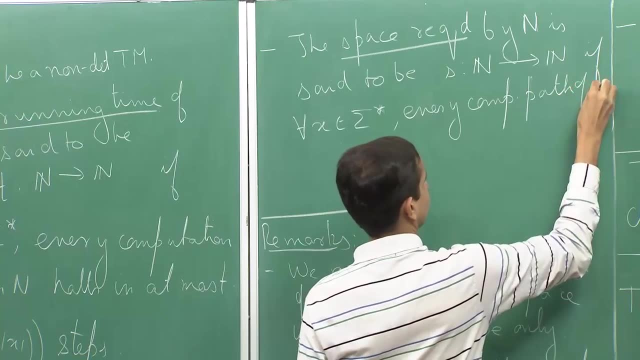 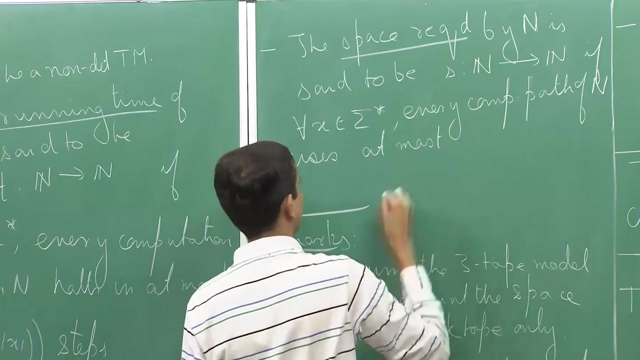 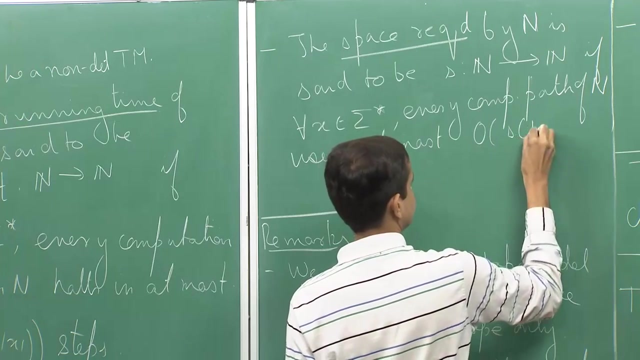 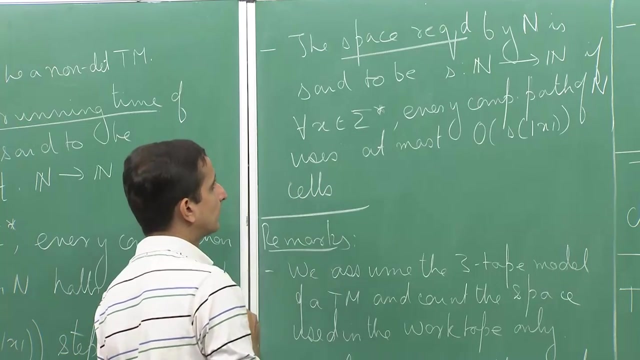 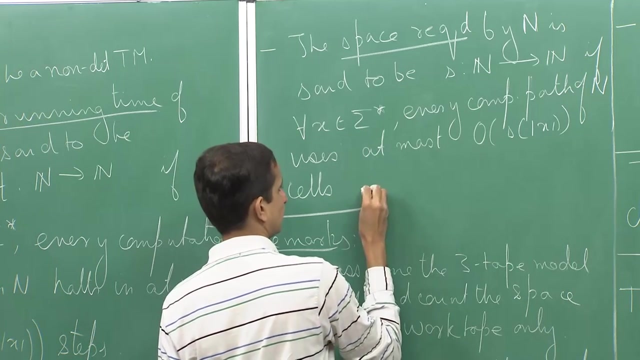 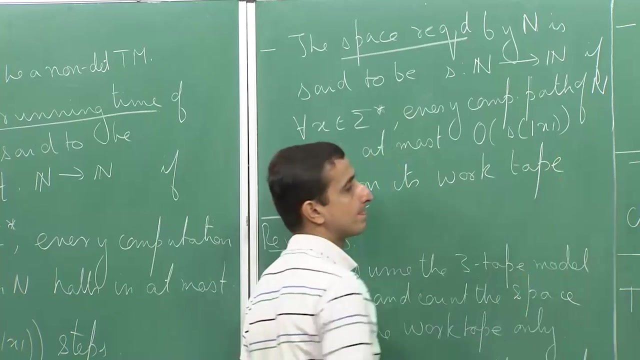 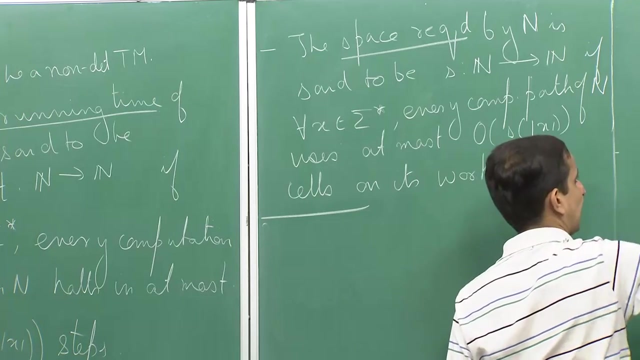 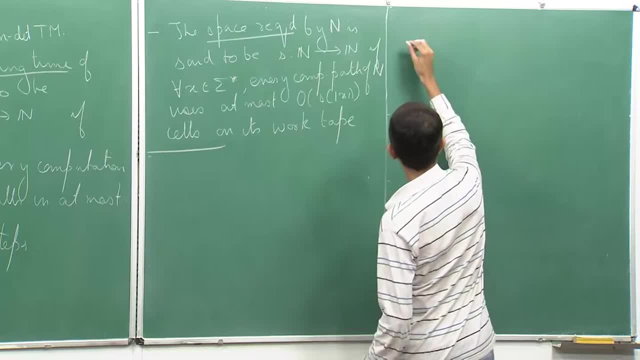 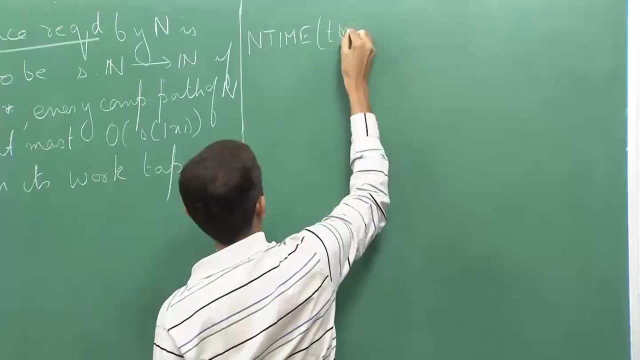 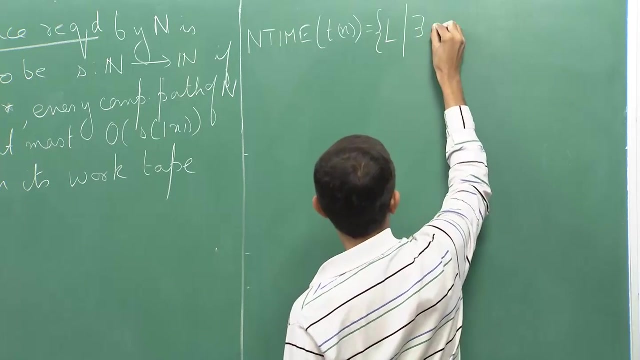 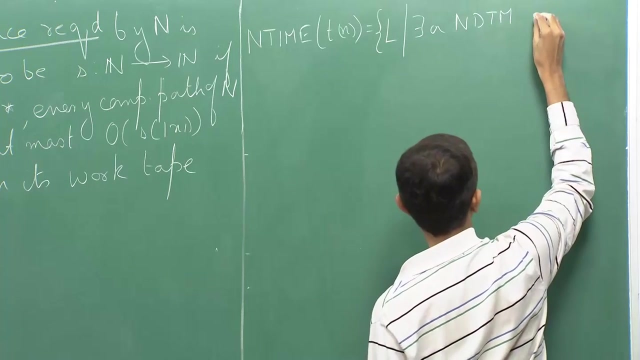 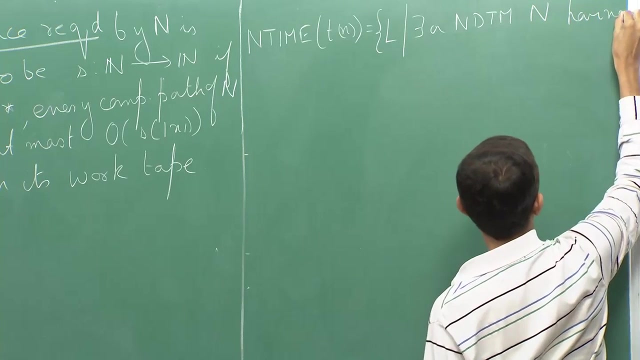 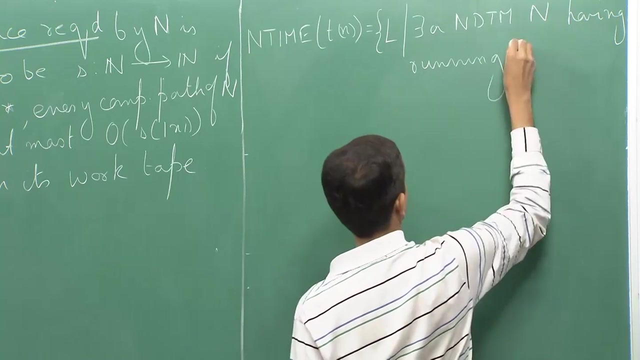 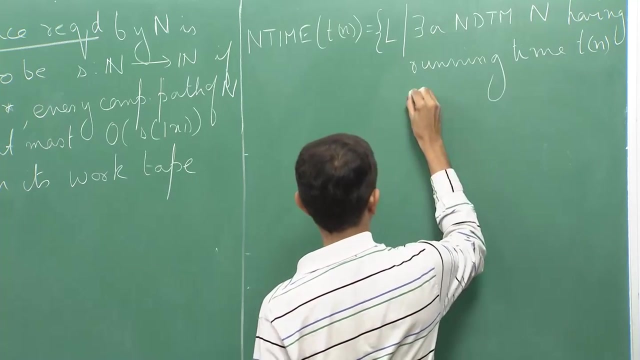 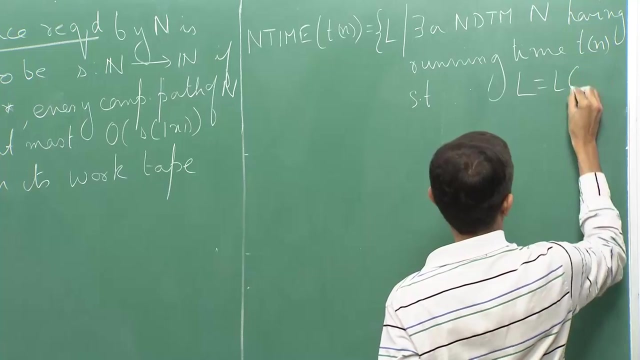 Ok, So we define the class n time t of n as the class of languages, L, such that there exists a n dtm non-deterministic Turing machine. n Ok, Having running time t of n such that L equals L of n. 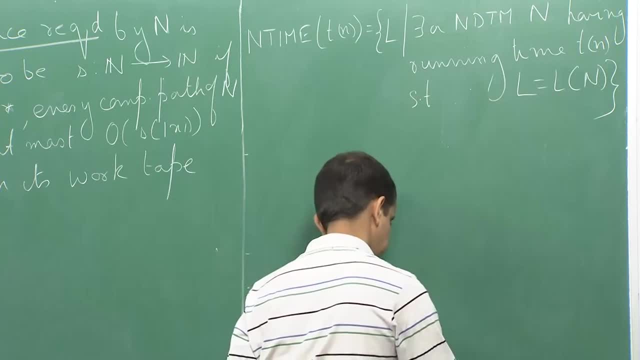 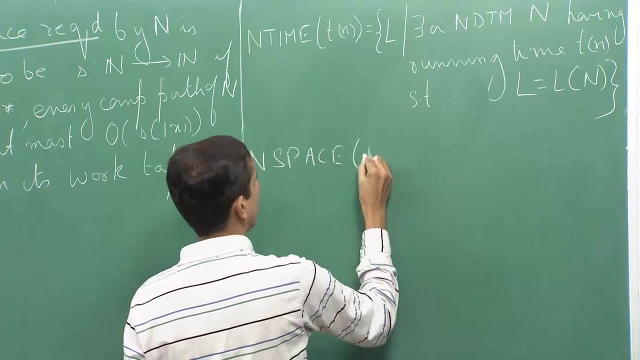 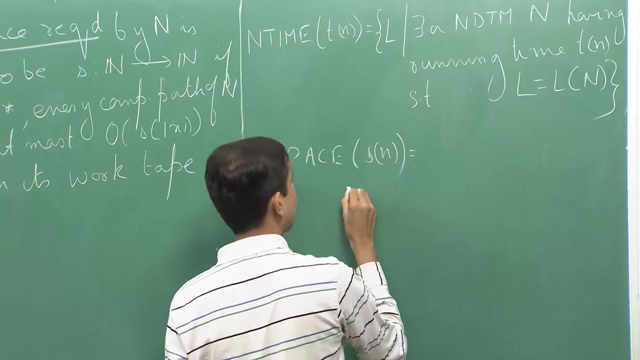 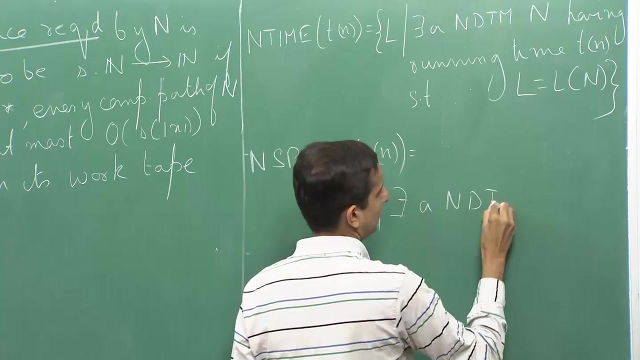 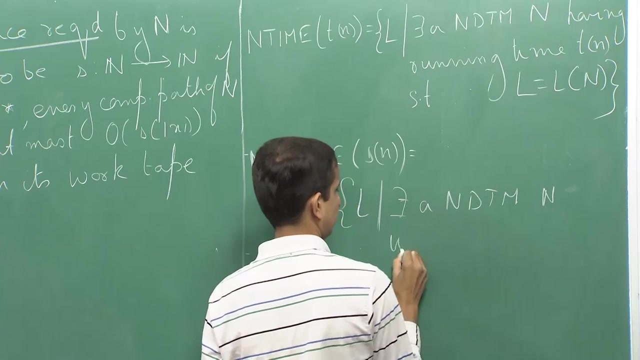 Ok. Similarly, n space S of n is defined as the class of all languages. L, such that there exists a non-deterministic Turing machine, n using S of n as the class of all languages. L, such that there exists a n dtm. non-deterministic Turing machine, n using S of n as the class of all languages. 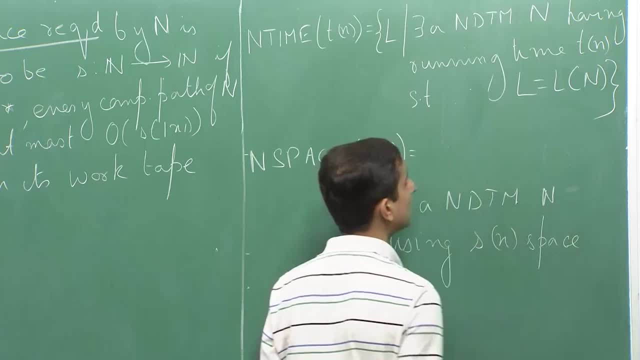 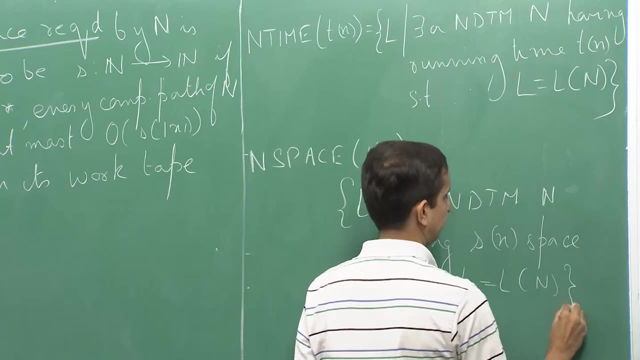 L, such that there exists a non-deterministic Turing machine, n using S of n. Finally, further, every loin material is set as like n of n, et cetera forever. every norm is set as like and n interior of the basic code: n, t of n. 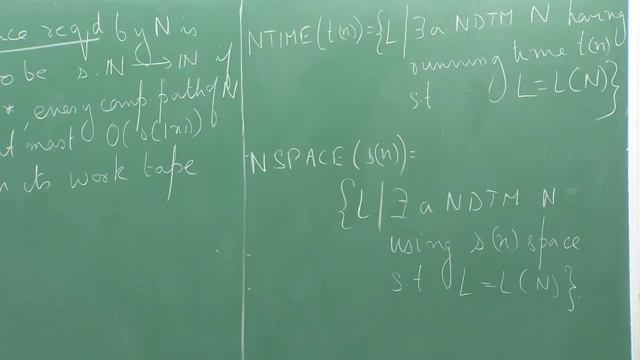 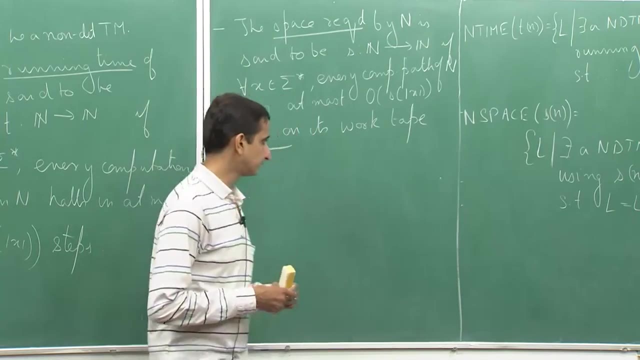 Ok, So this is how we define deterministic time and space classes, as well as non-deterministic time and space classes. Ok, So now let us look at some specific deterministic and non-deterministic classes. In fact, we will define witchут, tri, multiple interlets, totechnoline, two distribution. 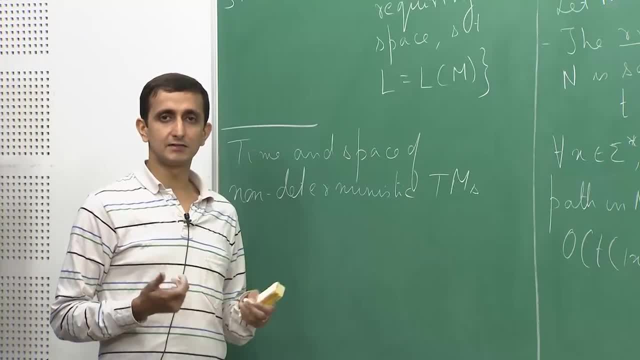 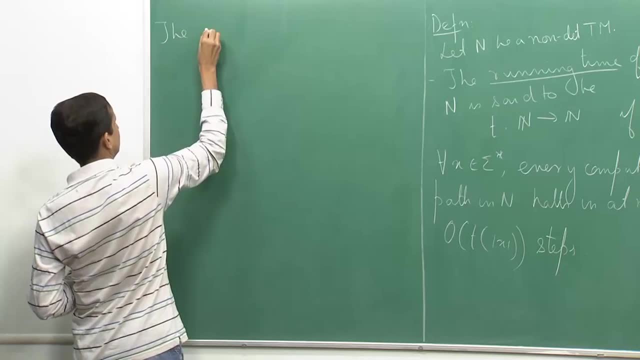 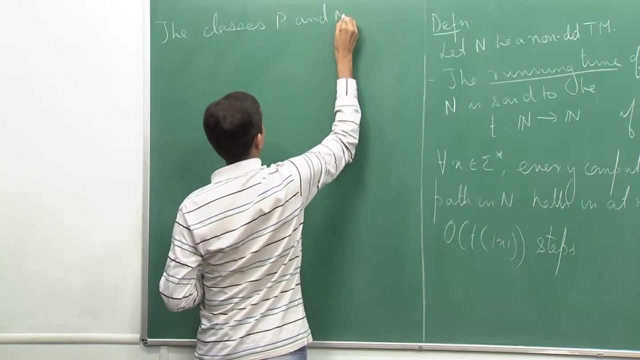 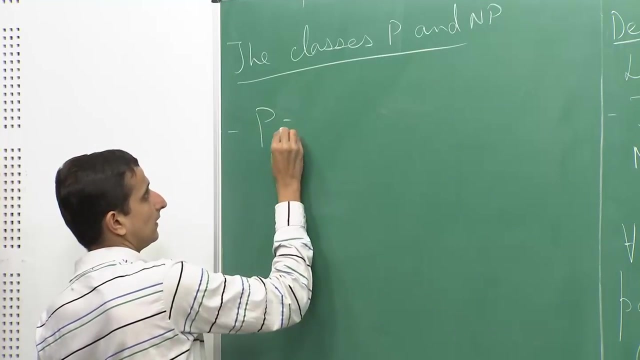 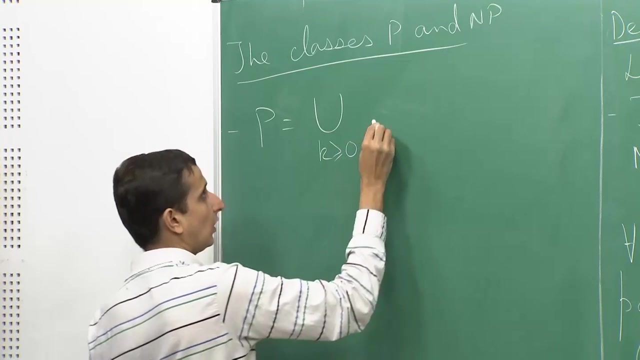 Containment of gift. chrism Plot. sweetIG T lab define the popularly known classes P and NP, So the classes P and NP. so P is defined as the union over all k greater than or equal to, let us say, 0 of time. n raise to the power. 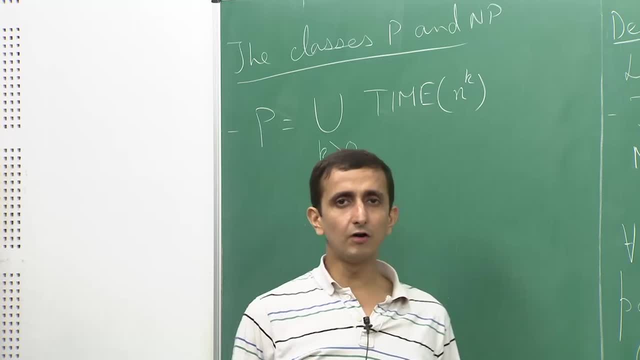 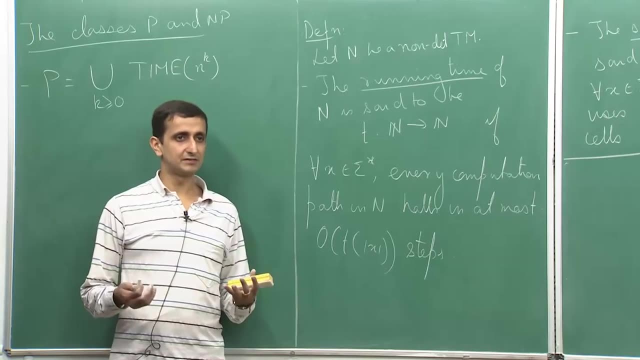 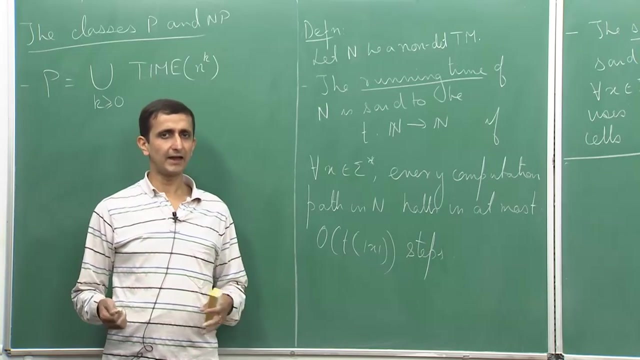 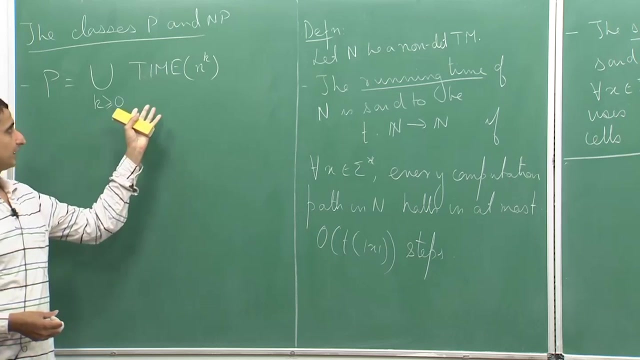 k. So look at all problems that have a running time, either n to the power 0, which is constant, or n or n square, or n cube, or n to the power 4, and so on, And the class of all these problems is basically P, So basically all problems which have a. 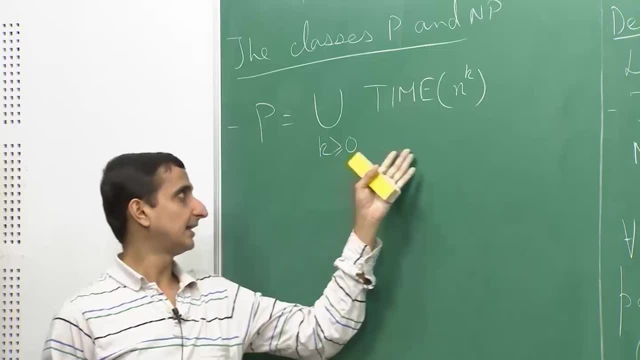 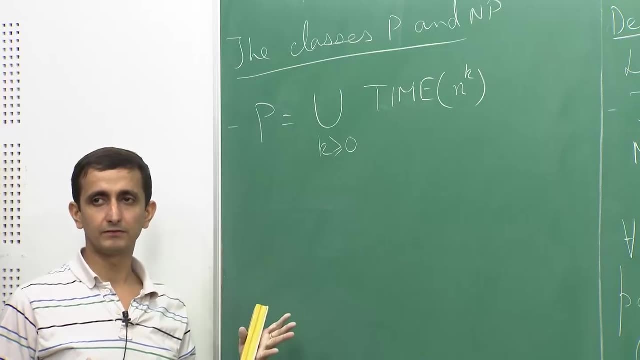 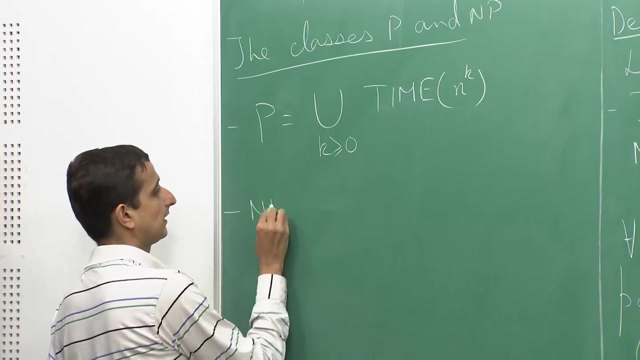 running time. that is polynomial. So if I say that a language belongs to P, that means it belongs to n to the power k for some k, so it has for some constant k. So similarly, the class NP is defined as n to the power k. 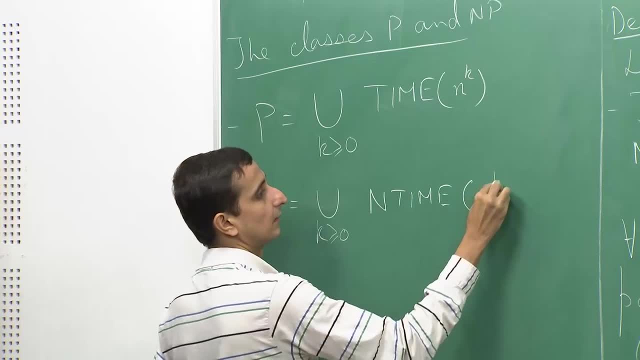 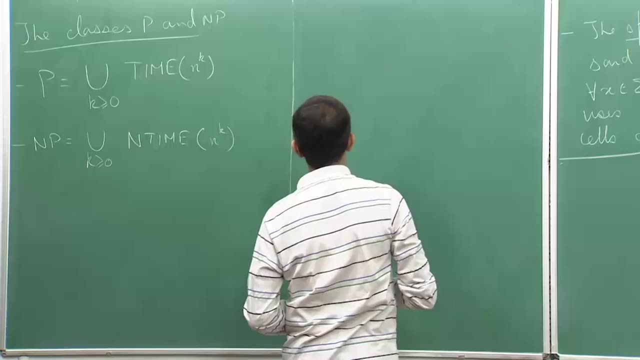 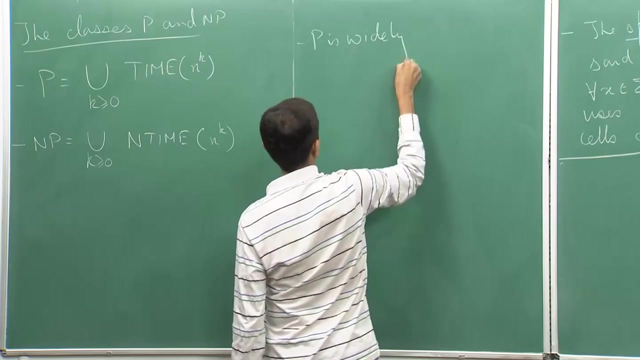 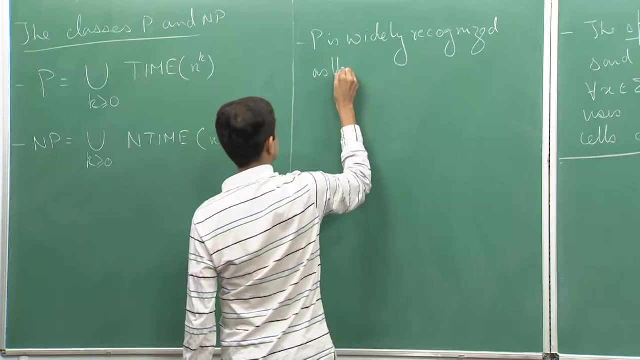 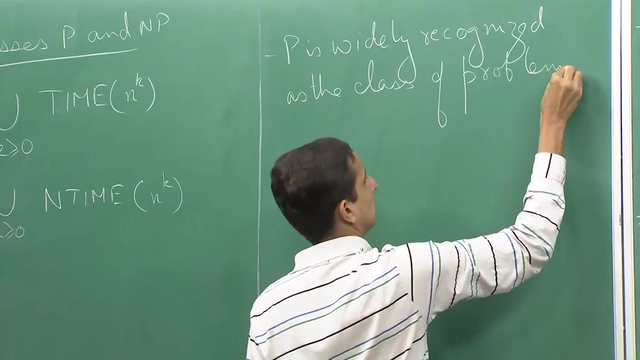 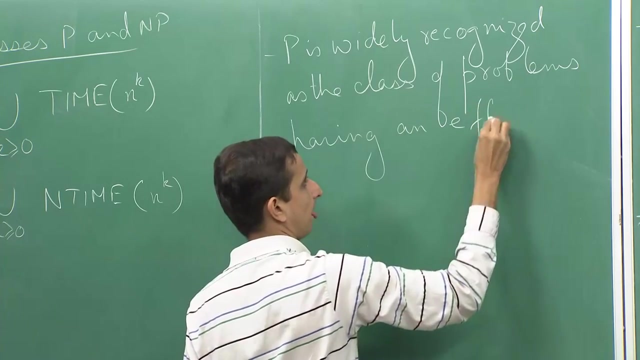 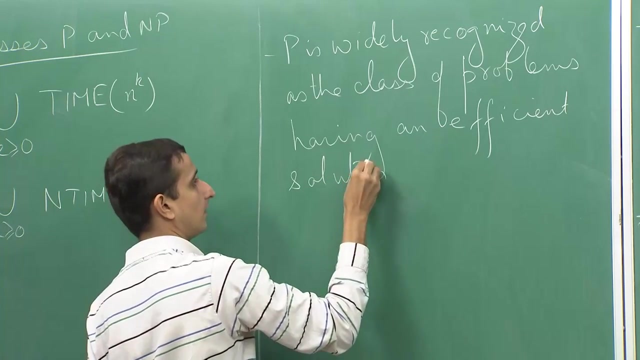 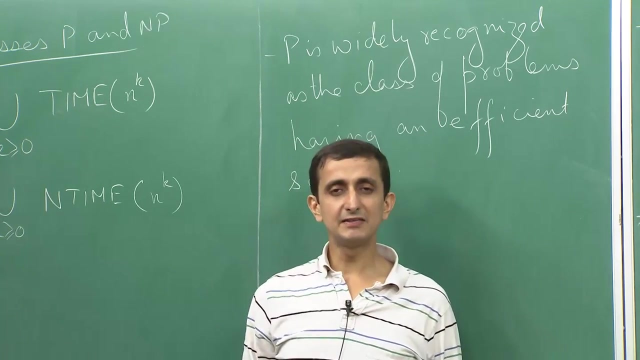 Of n, time n raise to the power k. So P is widely recognized as the class of k. So let us look at all problems having an efficient solution or algorithm. So, as I mean, it is widely recognized that if we have a problem that is in P, it means that we can actually 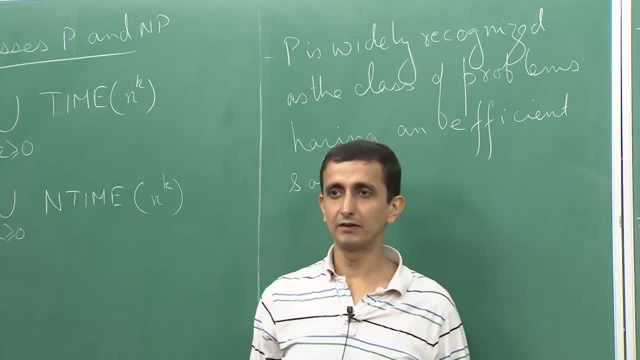 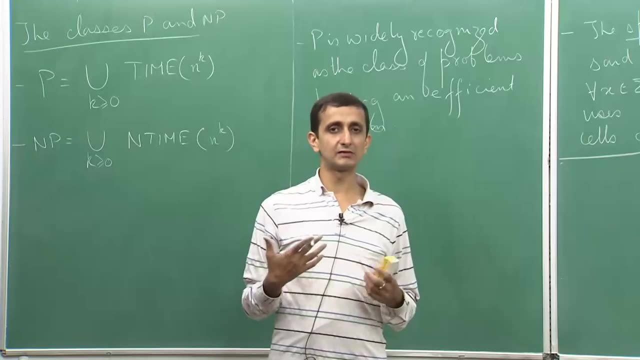 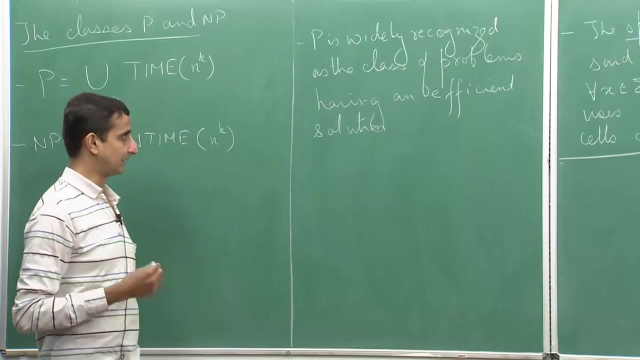 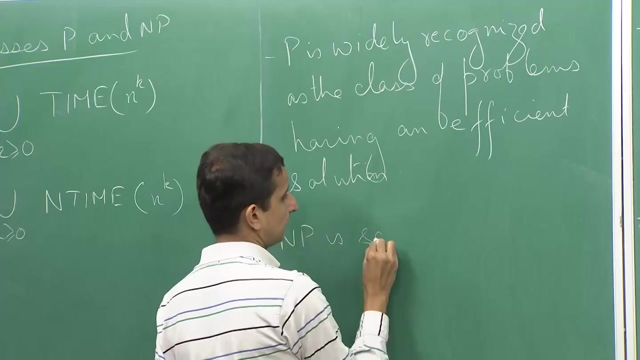 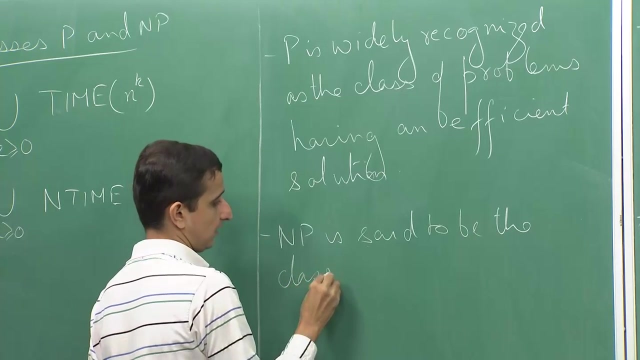 compute a solution to this problem in an efficient manner. For example, if we have a computer, we can actually write down an algorithm or a code for this problem that will produce an answer in a reasonable amount of time, so in quite quickly. On the other hand, NP is said to be the class of problems, So NP is said to be the class. 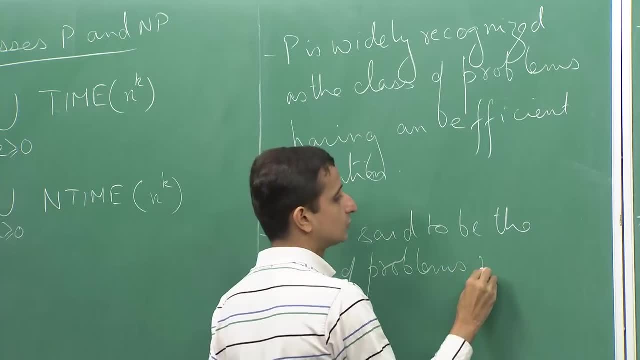 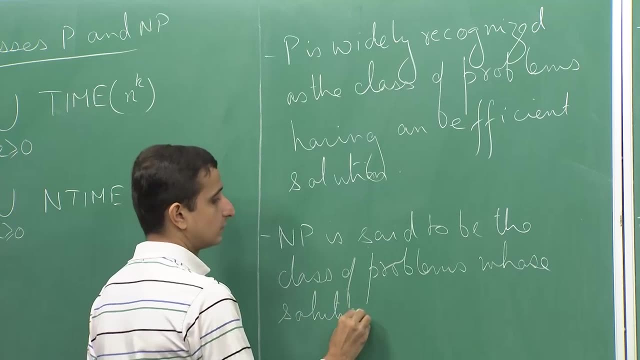 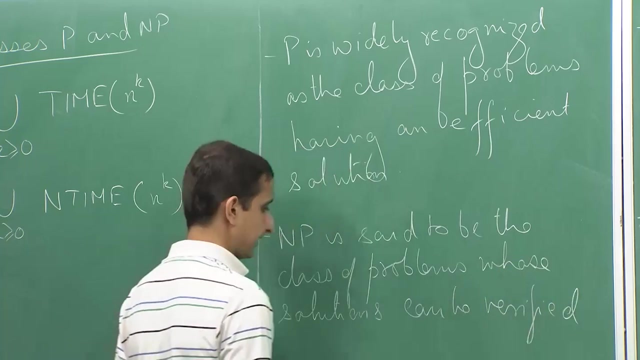 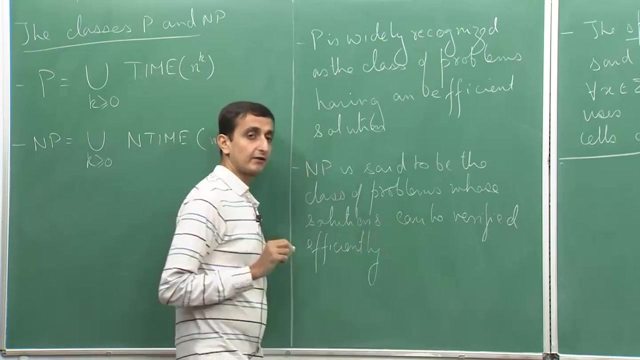 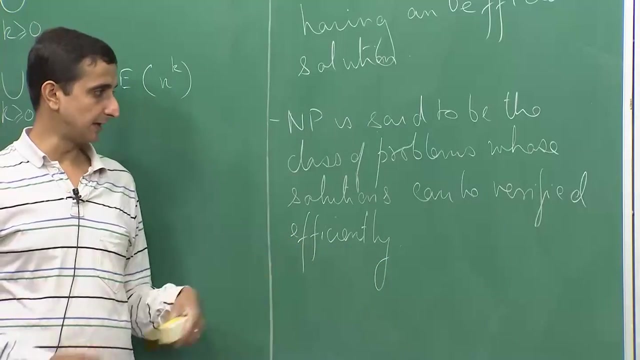 of problems. NP is said to be the class of problems. NP is said to be the class of problems. Np is said to be the n to the power k who's solutions can be verified efficiently. So actually, in our next lecture, we will give an alternate definition of Np, NP, which we 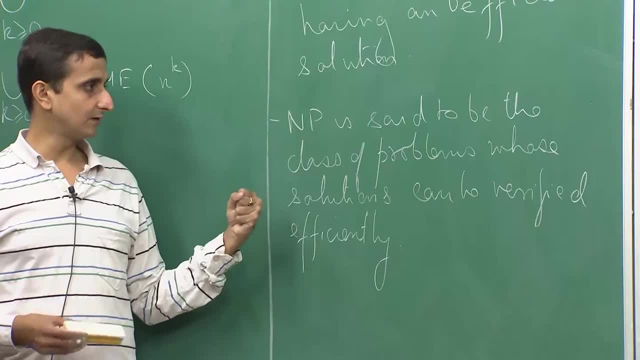 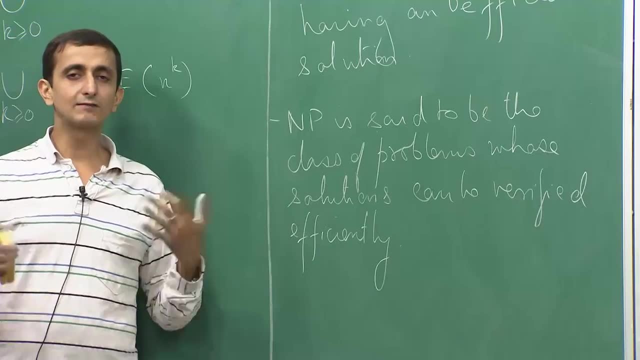 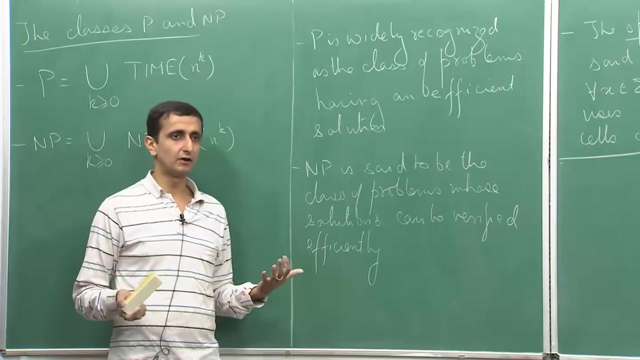 make this idea more clear, but I just want to give a perspective of what we mean here. So there are certain problems for which we can actually solve the problem in an efficient manner in some polynomial number of steps, such as matrix multiplication or given a graph. 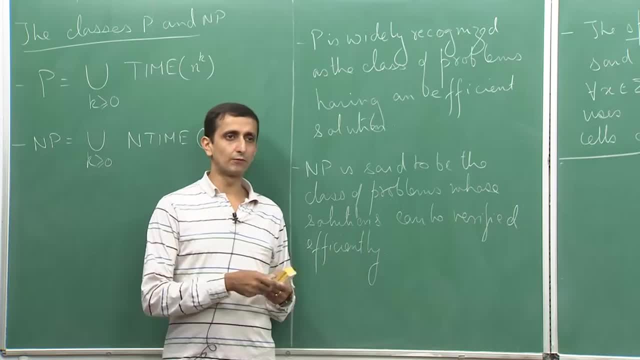 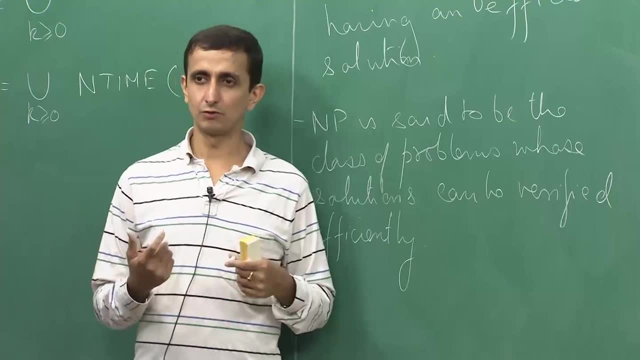 I want to find out whether I can go from one vertex to another. or, given an array, let us say, I want to find out the minimum element in the array, and so on. So these are the problems for which we say that there is an efficient solution. 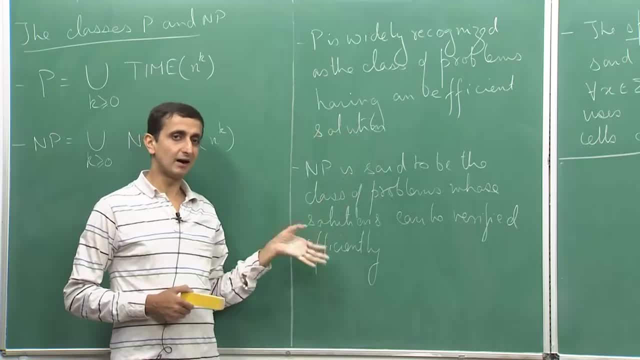 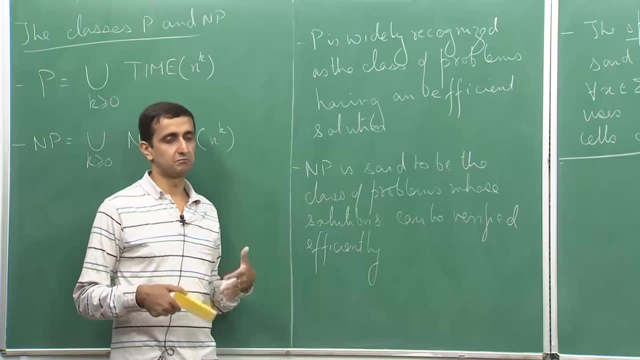 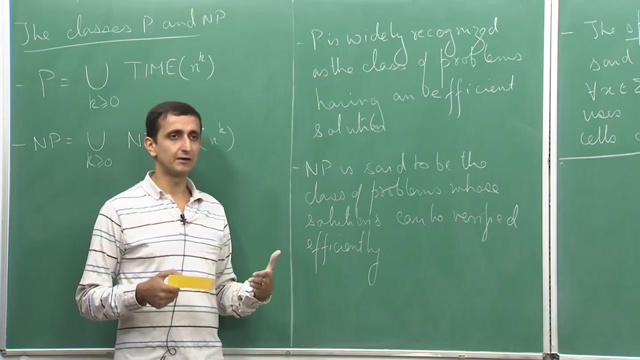 So these are the problems which are in P. There are some other problems for which it might be difficult to come up with a solution. So we do not know how complex I mean. whatever knowledge that we have, it does not seem likely that a solution can be computed efficiently. 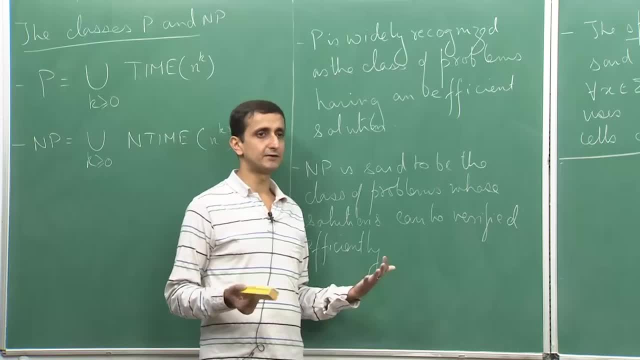 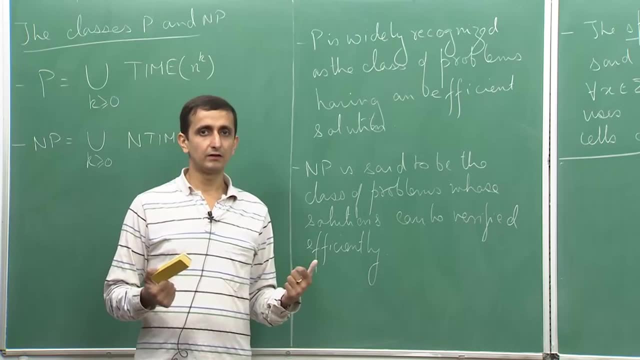 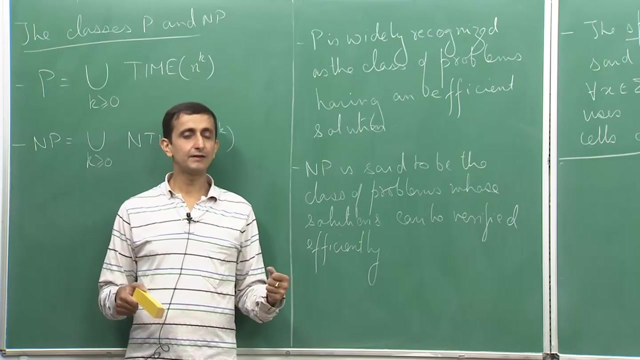 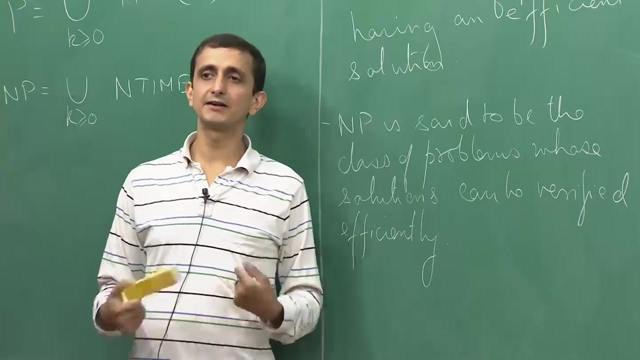 But if somebody gives us a solution, we can verify it efficiently. For example, think of the games, Sudoku. So in a game of Sudoku, if somebody asks you to solve Sudoku, it is more challenging than if somebody gives you a solved board of Sudoku and asks you to check whether it is a correct 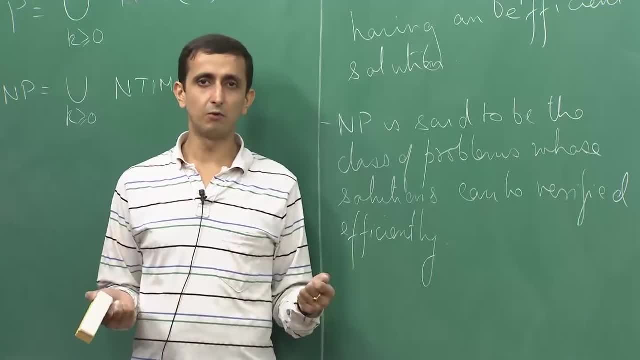 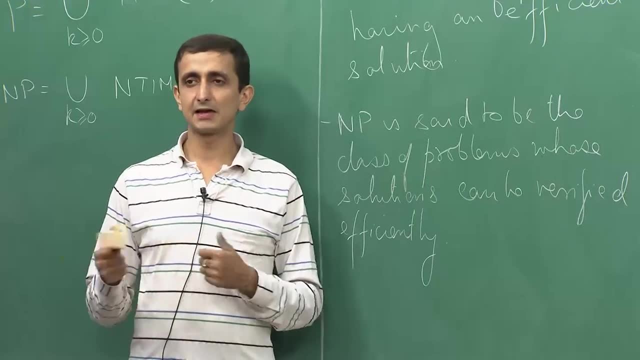 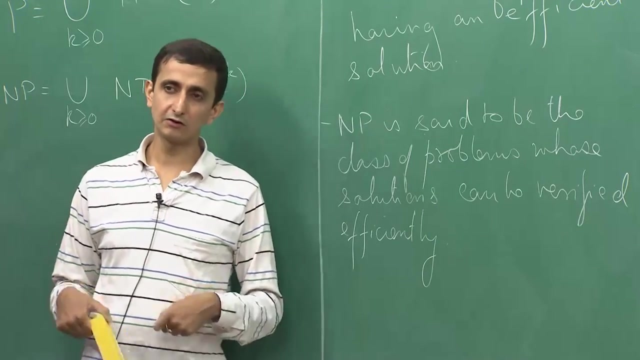 solution or not. If somebody fills out the boxes And then asks you, And then asks you whether this is a correct solution or an incorrect solution, you can very easily sum up and check whether the solution is correct or not. that is very efficient. But if you have to come up with your own solution, that is more difficult. 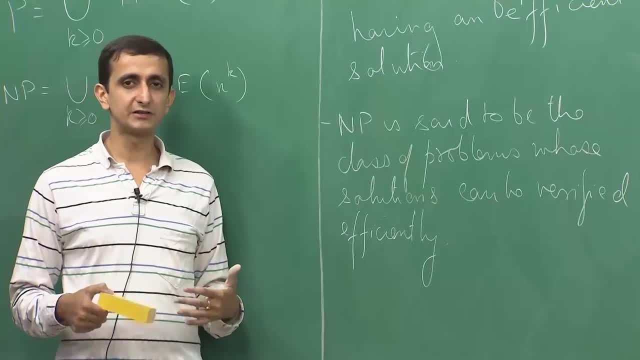 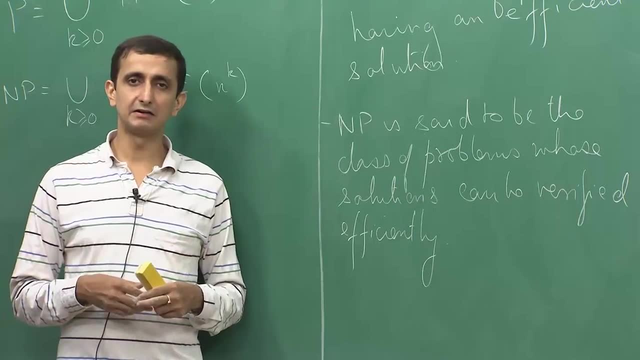 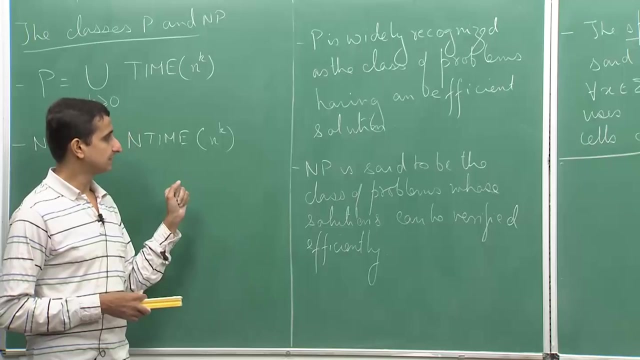 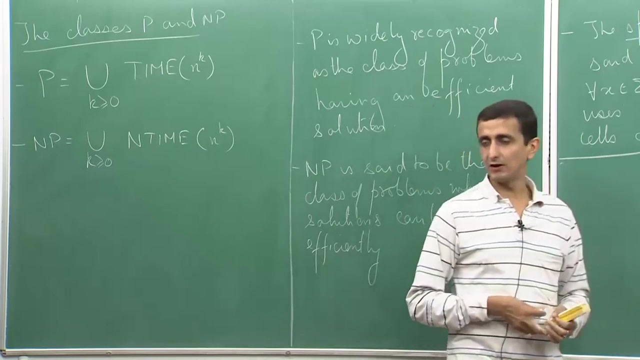 So there are other such problems for which coming up with a solution is, I mean, conceivably more difficult than verifying whether a solution is correct. So that is the, in some sense, the difference between P and the class NP. Okay, So next time we will look at more about these classes. we will look at more examples of problems. 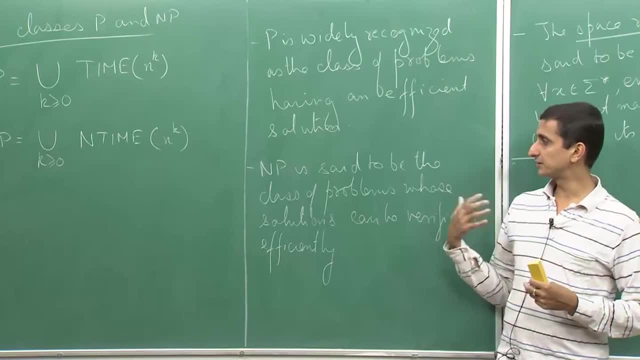 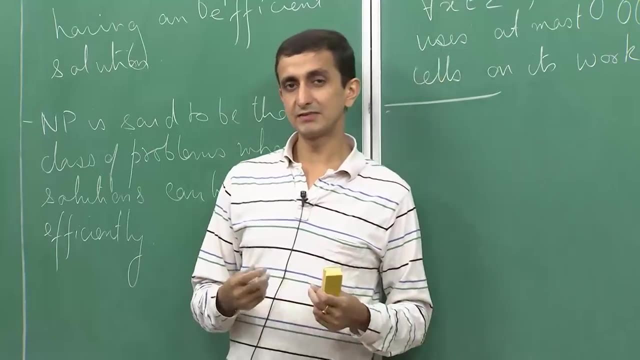 that are in P and NP, and we will also look at an alternate definition of the class NP which is more in line with this fact which I just mentioned, that NP is the class NP. Okay, It is a class of problems whose solutions can be verified in an efficient manner. 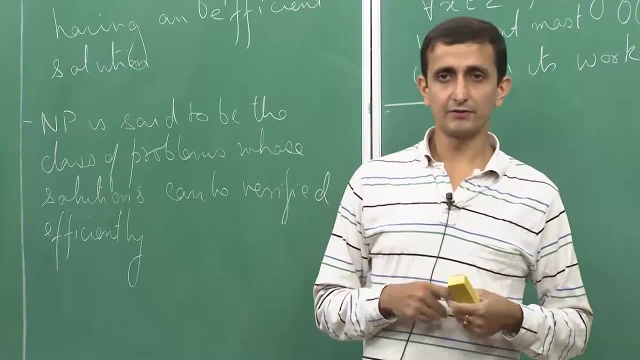 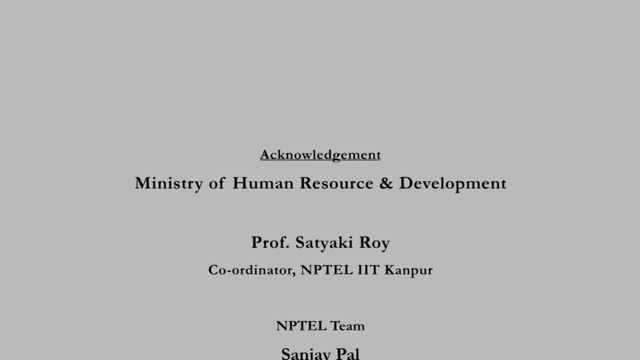 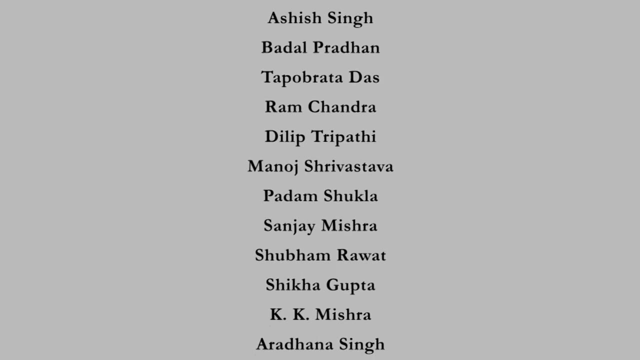 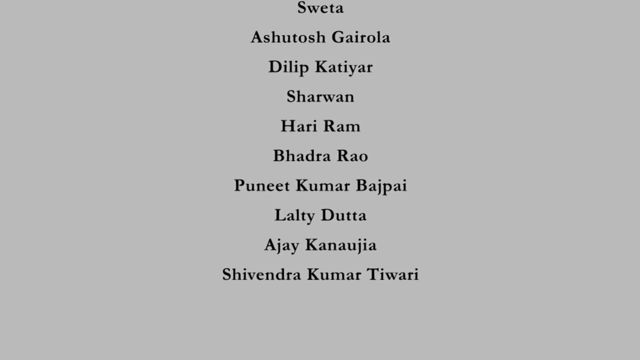 Okay, So I will stop here today. Thank you very much. Thank you, Thank you.